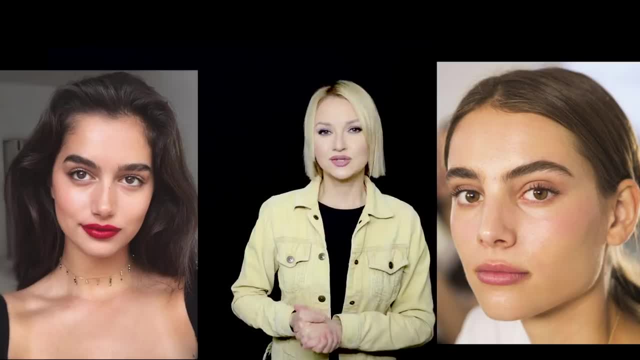 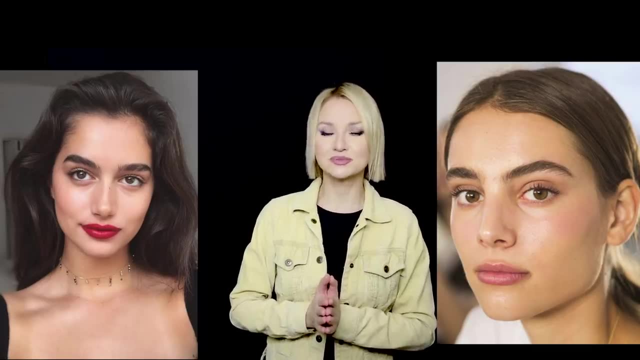 are seen from the distance and they are very clear and understandable. So first let's talk about brown eyes. So brown eyes is the most common eye color on our planet earth. It's about 50% of people have brown eyes and different shades of brown. Of course they can be super different, So they can be from. 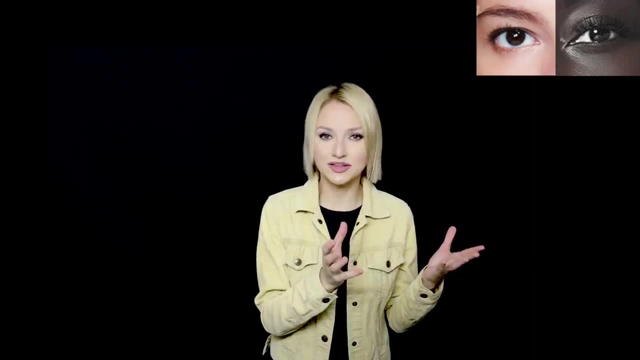 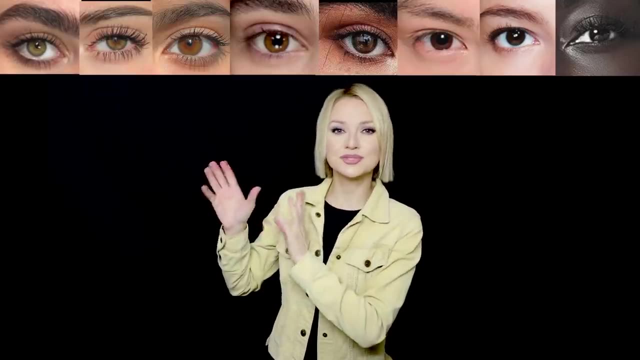 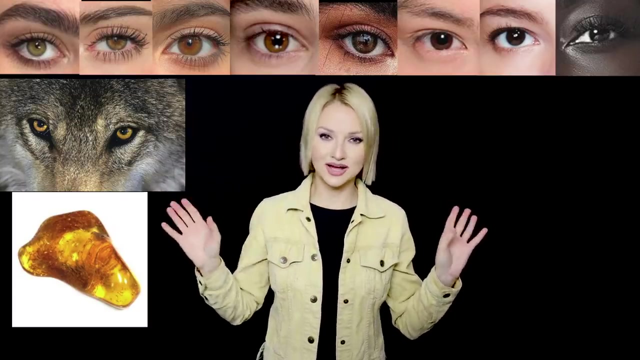 very black brown color so you can't see the pupil in there. It's just so so. so dark brown so it looks almost black. to the lightest brown, which we call sometimes wolf eyes, amber eyes or yellow eyes. All that spectrum is within brown eyes. All those eyes look different in combination with 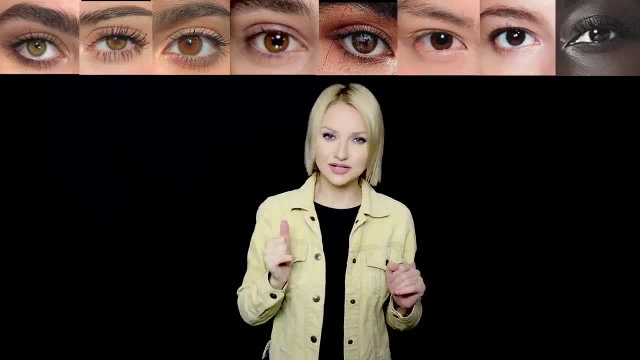 other features of a person. Everybody has whites of the eyes, right? Some people's whites are a little bit less contrasted, less white and bright, but they're still kind of white, right? Every person has different amount of contrast between their pupil and iris with the 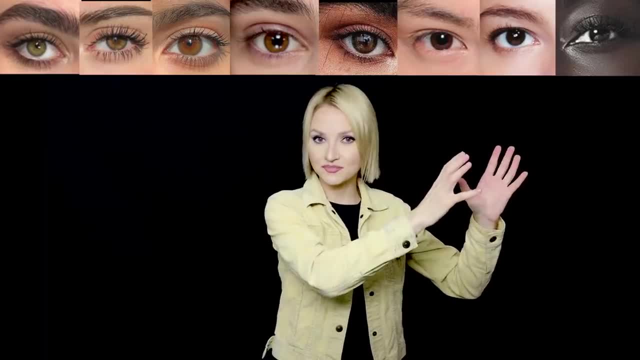 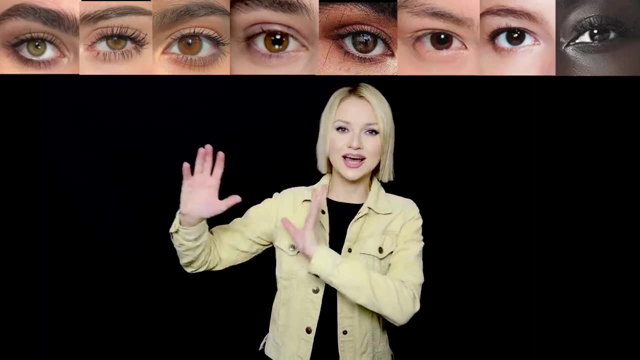 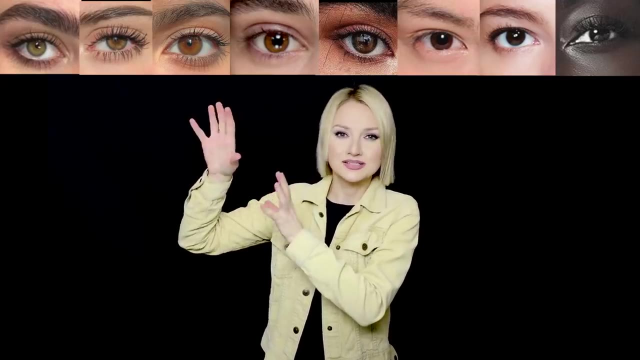 whites. So the darker the color is, the more contrast there is with the whites of the eyes, The more contrasted that area on their face looks. Now, if we talk about lighter eyes, the lighter the eyes, the less contrasted they're gonna look. with the whites, Finally, they look like glass very. 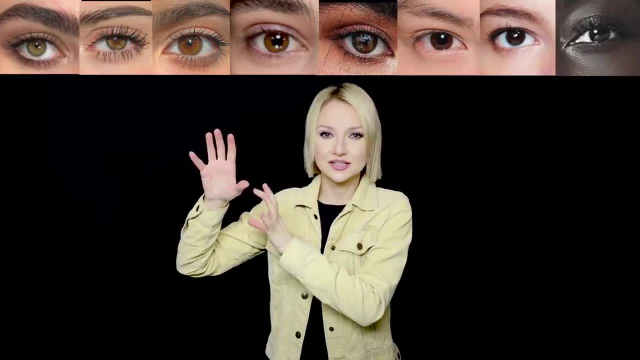 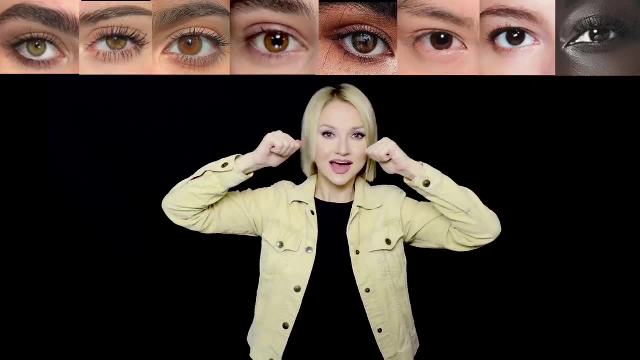 glossy, shiny and sometimes transparent, Like the lighter the eyes look, the more kind of transparent they look. It looks like the light goes right there to the middle of the head, like through the tunnel, When you look at yourself or when you look on people around you if you want to analyze their features. 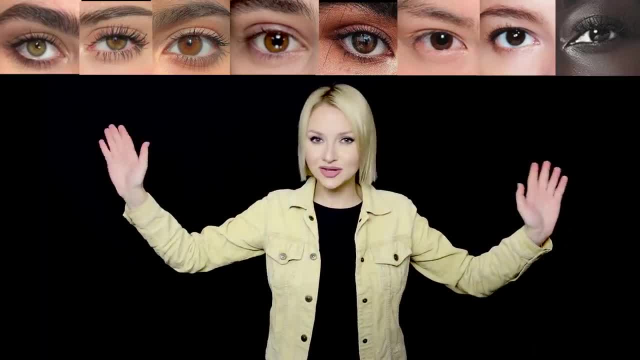 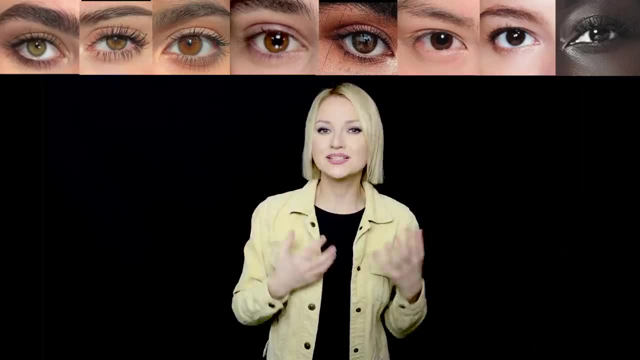 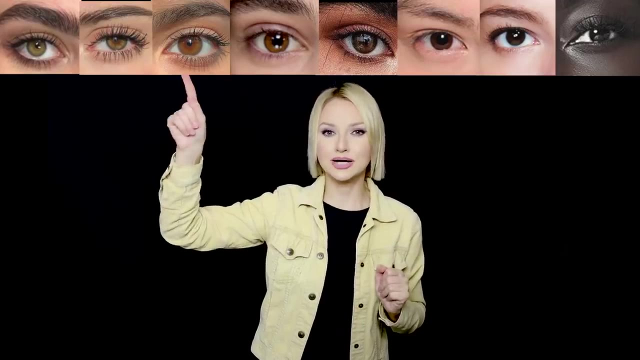 you should be able to say where in the darkness or lightness scale their eyes are. It's actually influences on the palette they look the best on. If person has many dark, dark, dark colors in their complexion, the less heavy dark colors will look on them. Of course, if we compare yellow eyes with 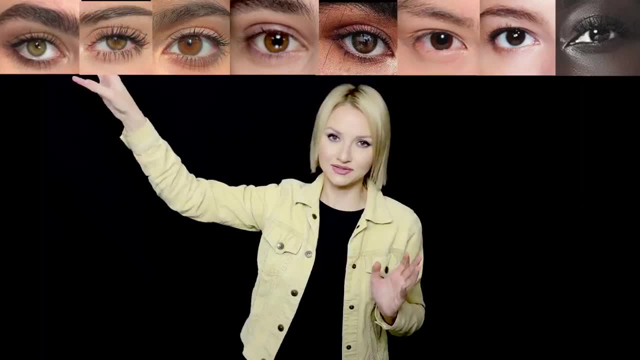 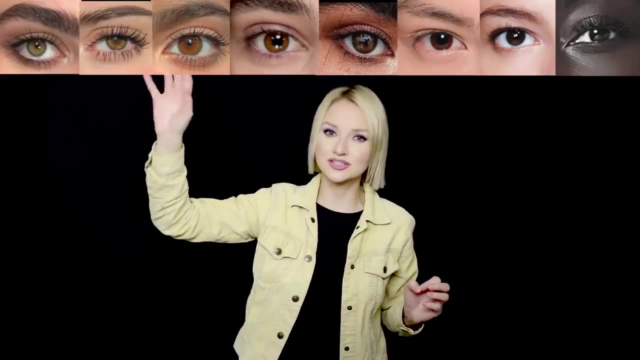 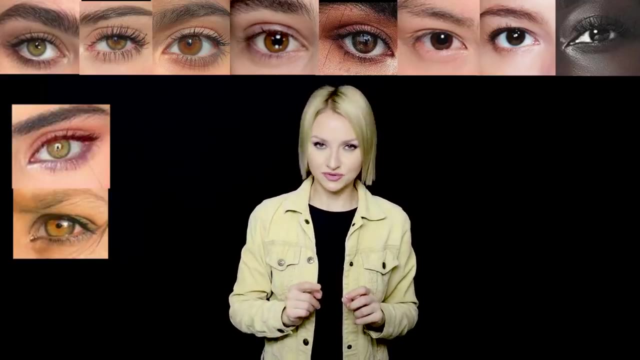 very light blue eyes. light blue eyes probably gonna be even lighter than that. See, amber eyes already consists some black, so it's slightly on the darker side still. Especially if lighter eyes have the frame around their iris, then they're going to be much more contrasted with the whites. 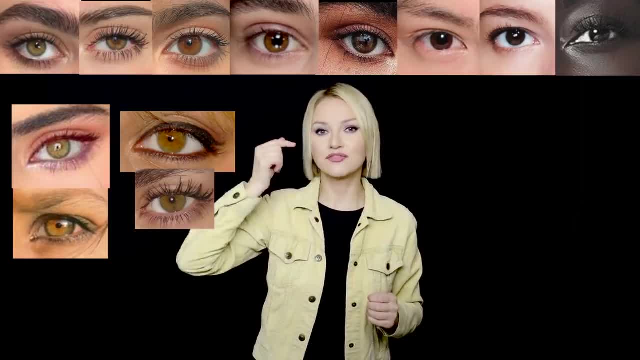 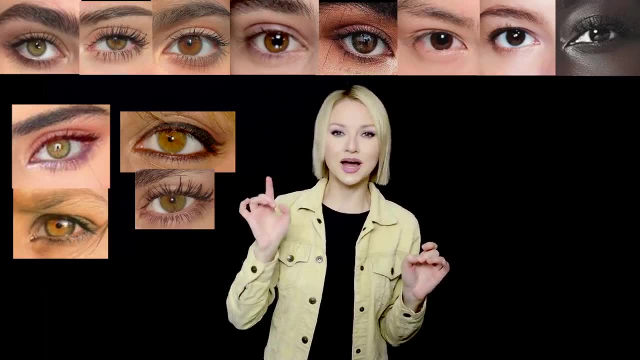 And this is another thing that we should consider, because if they don't have that frame, that lighter color, lighter amber color, it kind of blends into whites, especially from the distance, So it will be a little bit harder for you to find those eyes in there. If we talk about 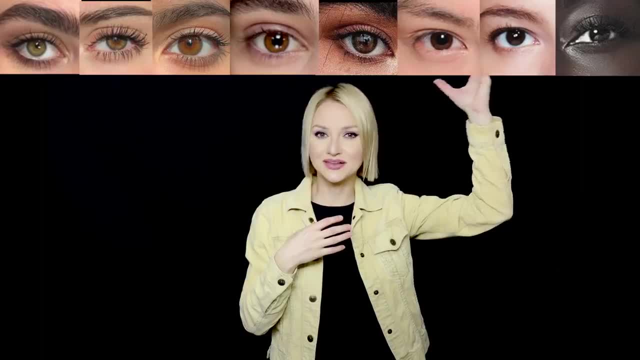 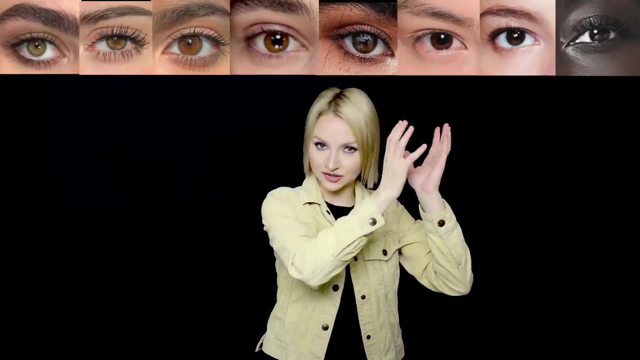 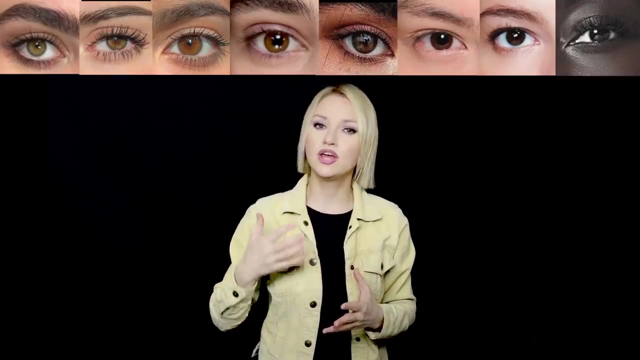 clearness of colors, brightness of colors. you can notice that those black eyes, that brown eye, reddish brown eye, very bright, intense color here, those are pretty understandable from the distance. right, You have no doubt about it, This color is pretty clear, understandable. 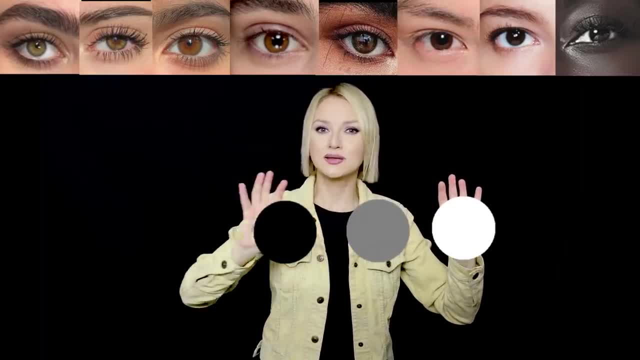 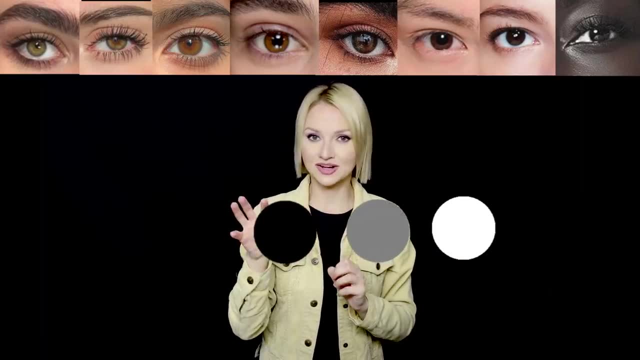 it's pretty bright from the distance. If we talk about white, gray and black, which of those this one contains the most? Of course, black right Mostly has black color. It doesn't have as much gray color, otherwise it would look lighter, slightly muddy and uncertain, And then it's not. 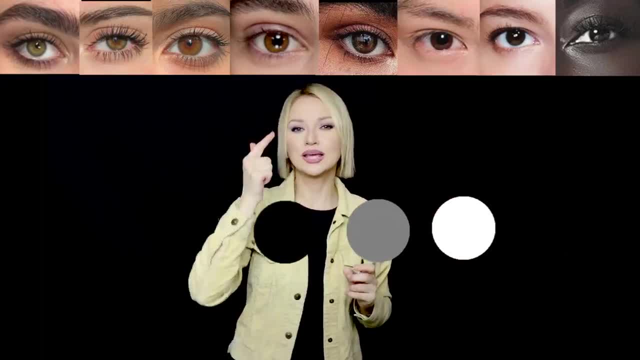 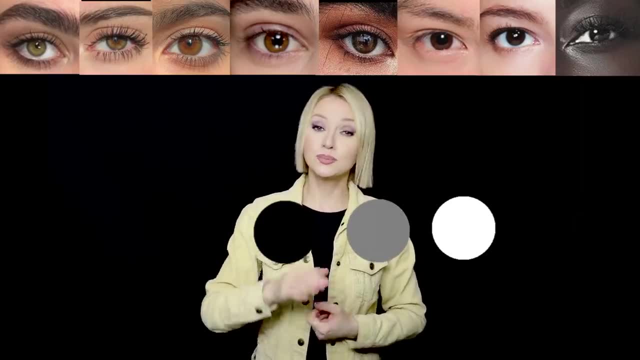 whitish as well, Because it's super dark right. You also can sometimes imagine whether it contains more white, gray or black. That will be a great training for your eyes. You will be a pro with that. So if we go to the lighter brown color- and it's still pretty clear, it's still pretty understandable. 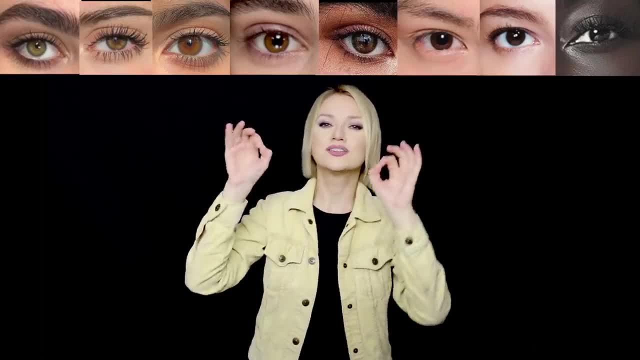 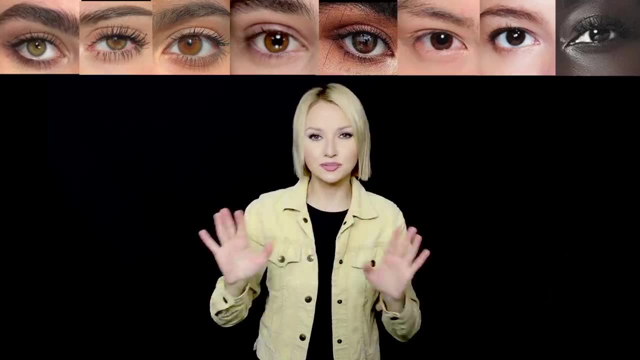 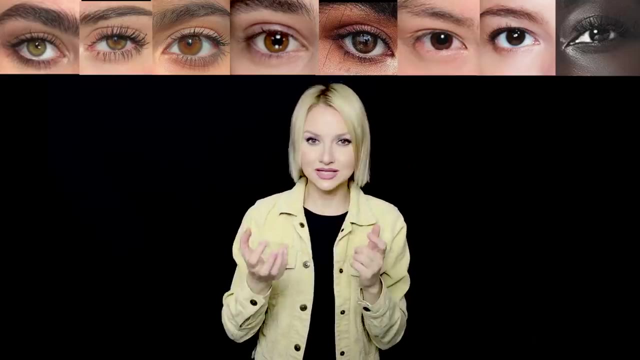 from the distance. It doesn't have those additions of colors, slight dots, zigzags of different colors, any rings or halos around the pupil. No, it's just very plain clear brown color. If we talk about lighter brown eyes, they have more and more yellow color to it and less intense black. So when we look on, 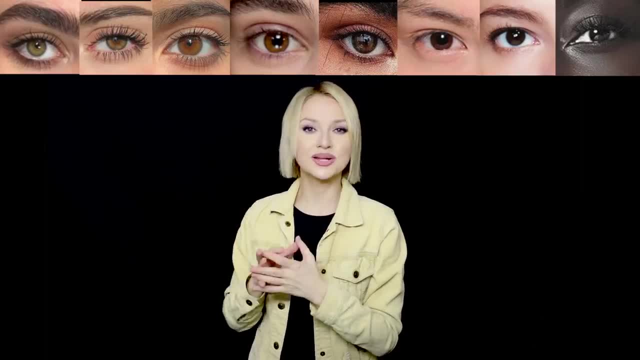 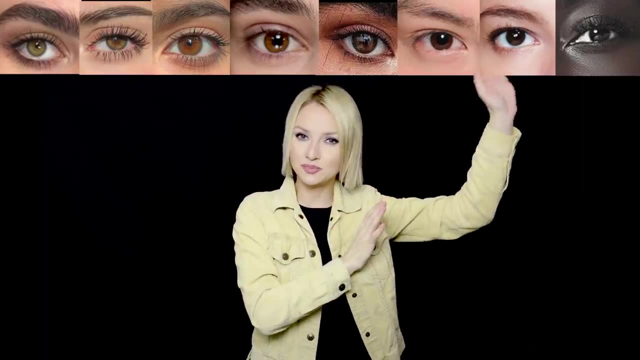 them. they look warmer for us and they also look pretty understandable for us. They look pretty clear, they look pretty intense and they look warm. So normally, very often, people with black eyes or somewhere around here- many of them have cooler undertones and many people having those- 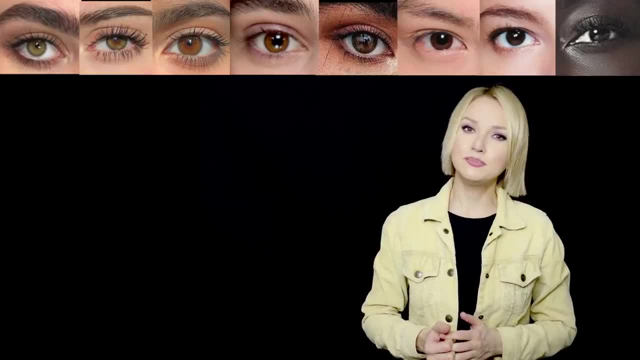 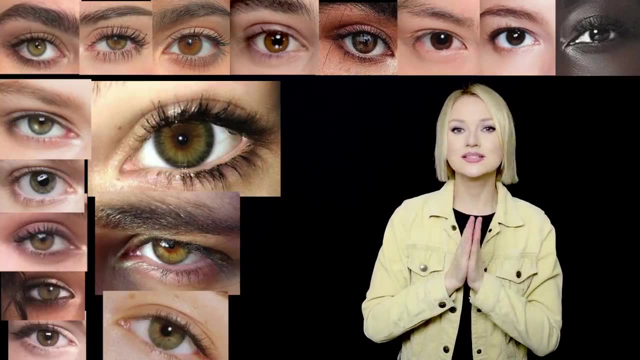 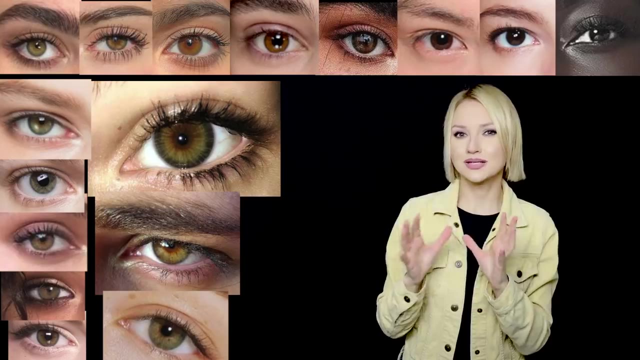 eyes have warmer undertones, Then very often people have mixture brown eyes with some other color, So we call that hazel eyes. Hazel eyes is eyes that have both brown color in them and some green. I also saw some hazel eyes now with green, but with dark, gray or blue color added to them. So 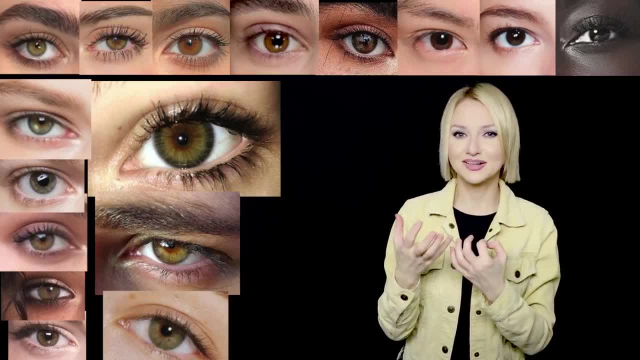 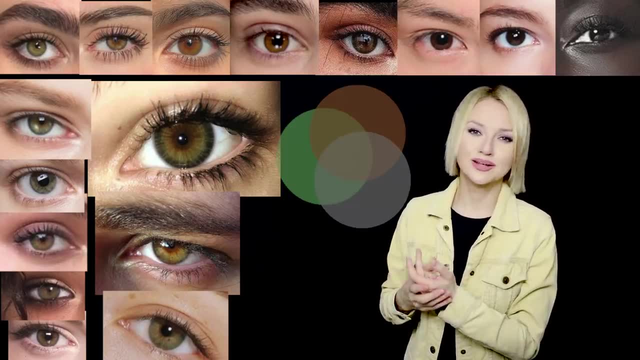 blue and brown again. that is some kind of muddy color added in them. And what is muddy color? Basically, mud is color that you can't name. That is normally a mixture of green, brown and gray, something like this. So this is a color of mud. I have pretty muddy eyes. 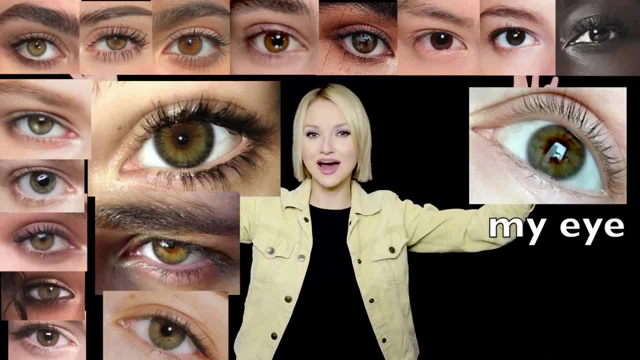 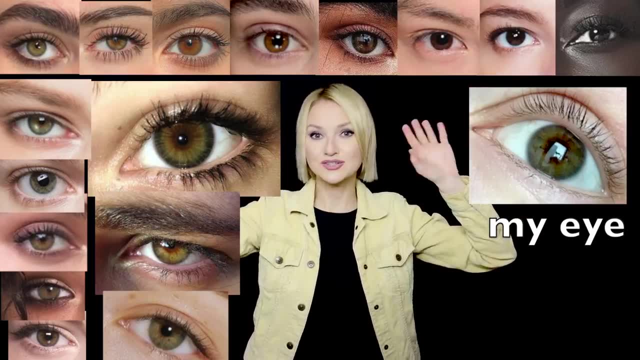 but because I don't have space in my eye, then I don't have enough space in my eye anyway. So these two colors are responsible for this. So we are doing a concept with my Whatever. So I have hazel eyes. If you look on the darkness of my eyes, my eyes are slightly on a darker side. 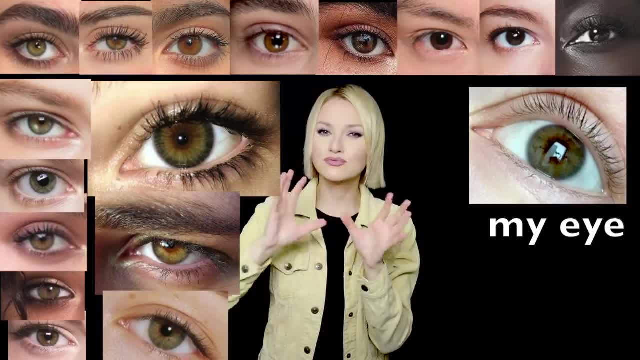 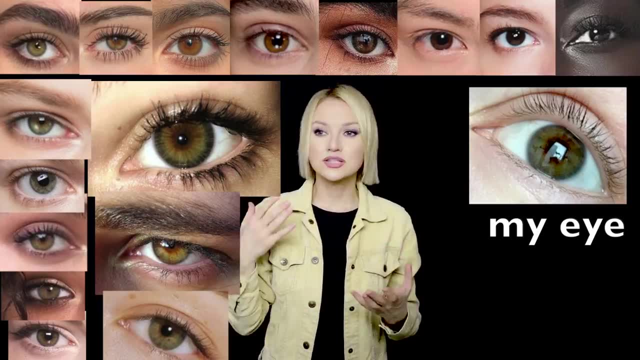 because my mom has very intense brown eyes. My dad has gray eyes so his grayishness was added to my mom's eyes just slightly and this is what happened. So in my eyes you can see some green, gray kind of colors added to the brown. so my eyes are not very black, dark, intense and very clear. 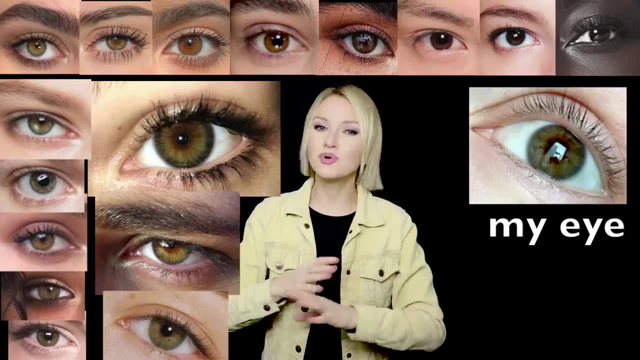 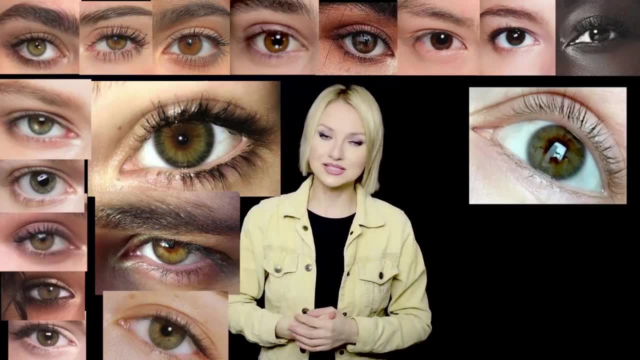 of my complexion, but my eyes are pretty contrasted- not the most contrasted if you compare myself to other people, but they're still on more contrasted side because i have pretty dark frame around my eyes and it's pretty contrasted with the whites. so i do look pretty good with some darker accents by 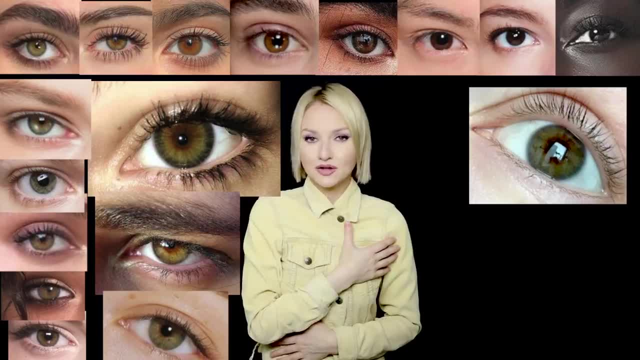 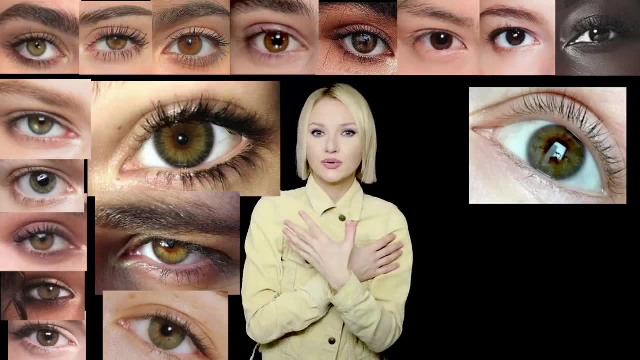 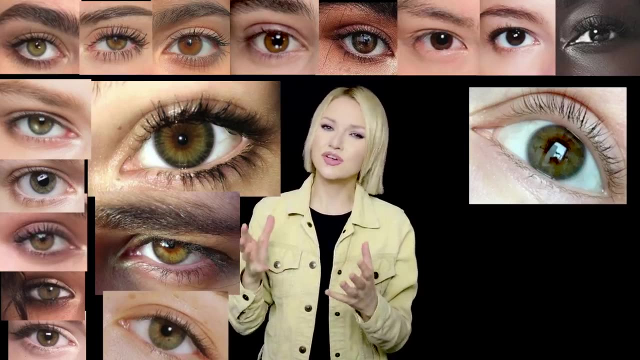 my face because so if i'm wearing something completely pale, and let's say i don't have any makeup, everything gets pale except for my eyes. my eyes don't have enough support, so they look very lonely. so the percentage of brown and green or brown and gray in hazel eyes, not very important. 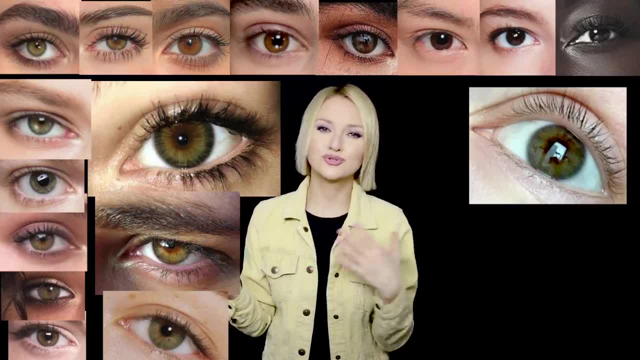 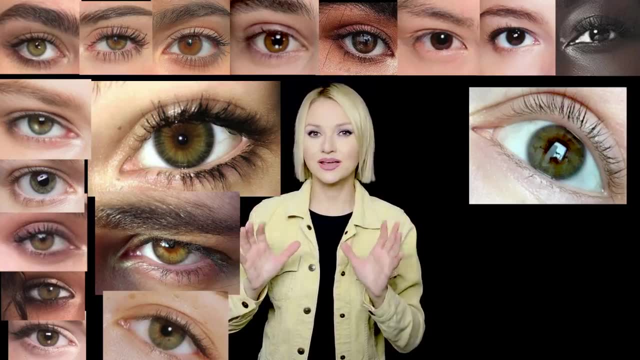 to be honest, because it's still not gonna be too warm or too cool. you're still gonna look slightly dull, slightly muddy, slightly ashy. it's still gonna look that way. it's still gonna look not as understandable that color. it can look slightly dirty, slightly muddy if i have a lot of purple. 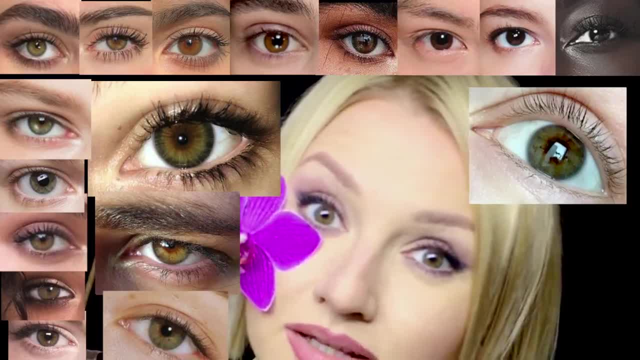 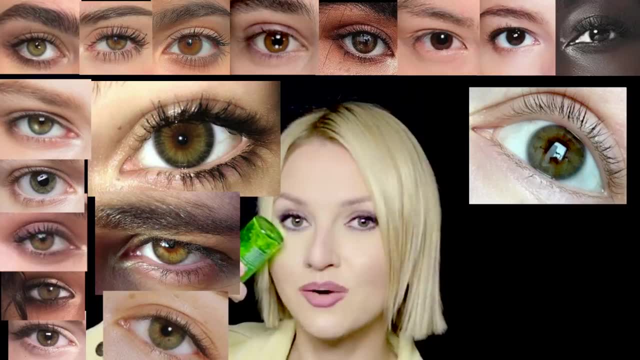 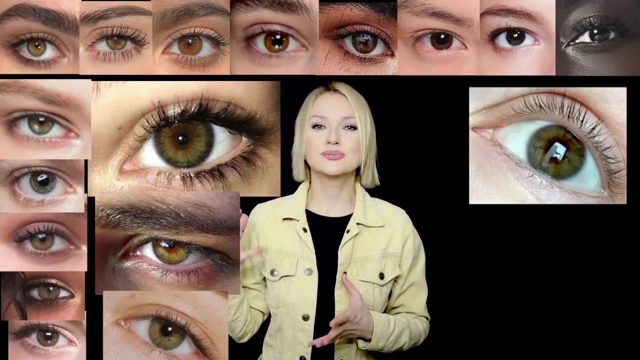 color. by my eyes they can look slightly greener, yellower, popping more. but if you place something green by my eyes you will be able to see that warmth more like brown colors more. so many girls with hazel eyes. they consider to be slightly on a warmer side, but they consider to be slightly. 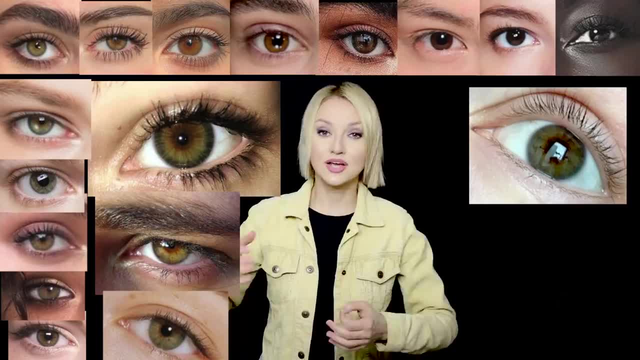 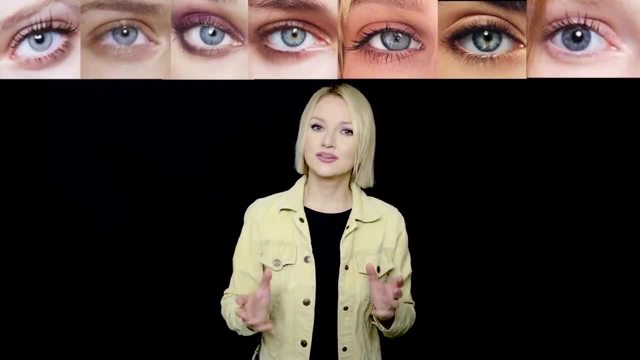 on a dusty side as well, slightly on a muted side, as opposed to clear colors, clear and very understandable from the distance. now let's go to blue eyes and again we have the scale from darkness to lightness. if we talk about clearly blue color without any colorful additions to it, let's say: 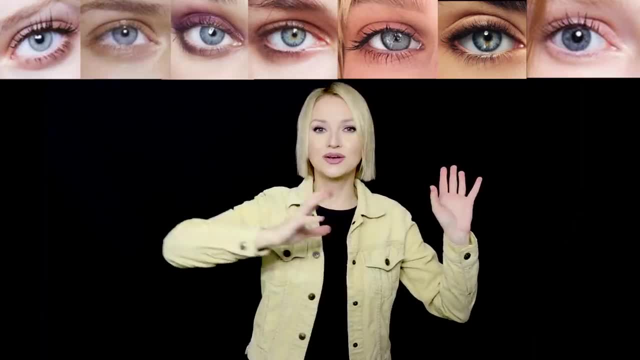 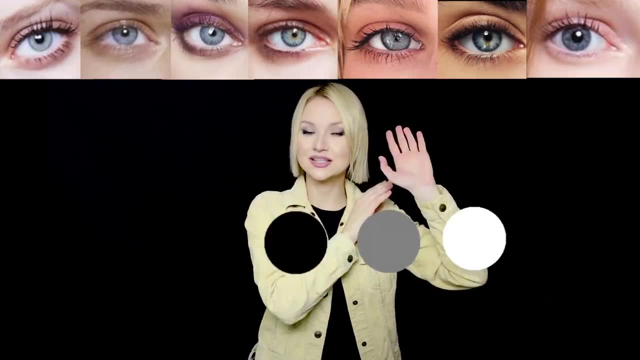 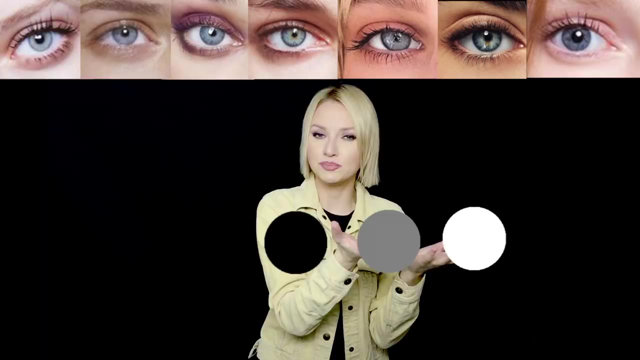 just plain blue color. so we have dark blue eyes. it goes right there to light blue eyes. if we imagine how much of black, gray or white colors added to them, you can see that in the darkest blue shade we have some black color added to that, even though it still has very clearly blue appearance. right, of course it's not. 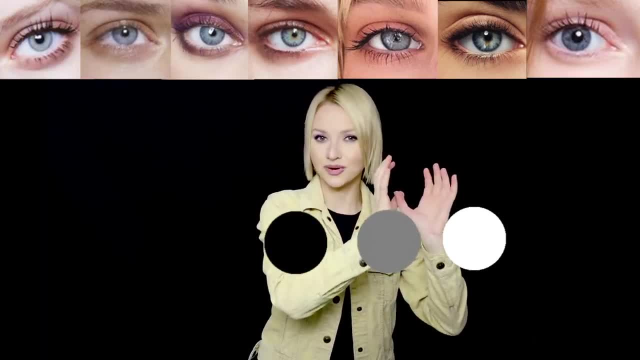 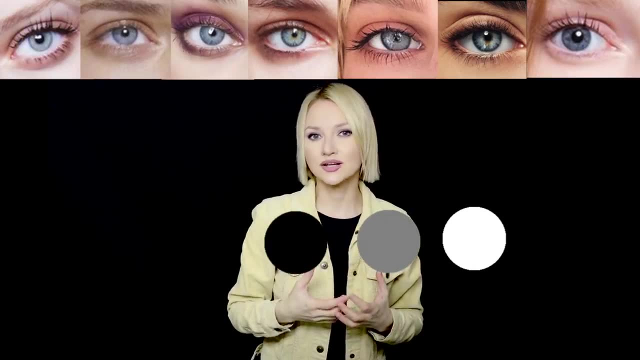 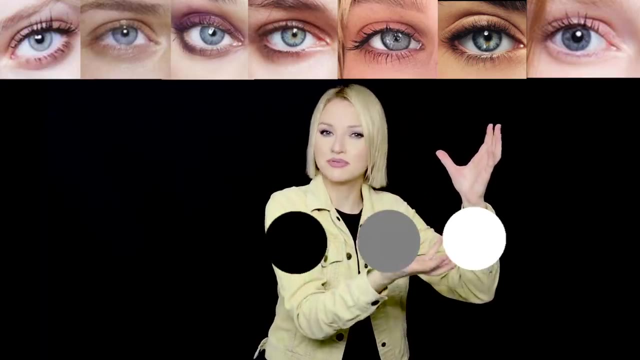 as intense as brown eyes. it still starts at the lighter point because we still have to find that color in there. blue and black, both added in there, and black is also clear color. it's not dusty and not muted, so it gives that brightness to those eyes, clearness, some depth in color and blue undertone. 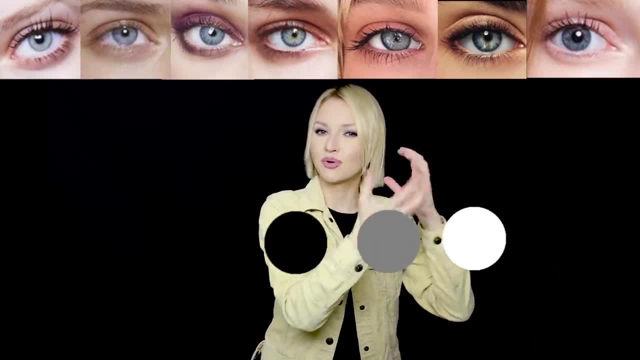 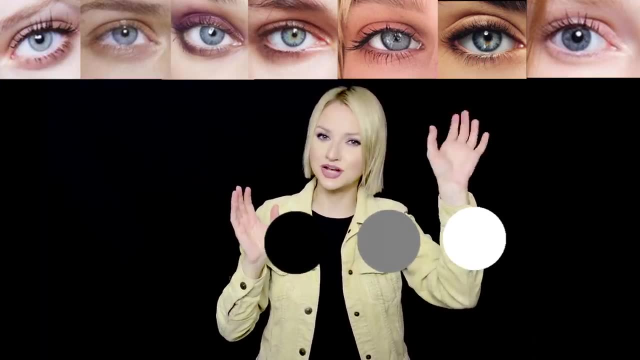 so many people have those eyes. that eye can really give some more contrast, more depth, into their appearance, even though they are light overall outside. but they still can have some darker blue eyes and, by the way, watch till the end because we're going to look on all those colorations of. 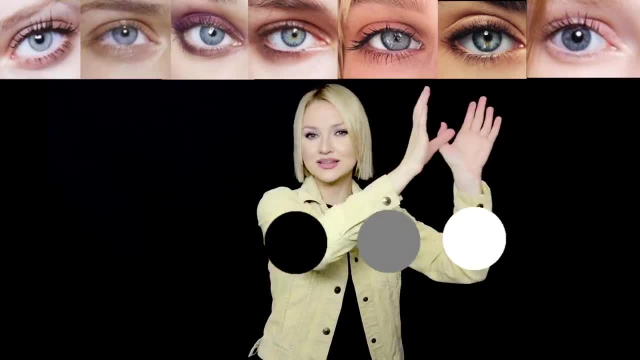 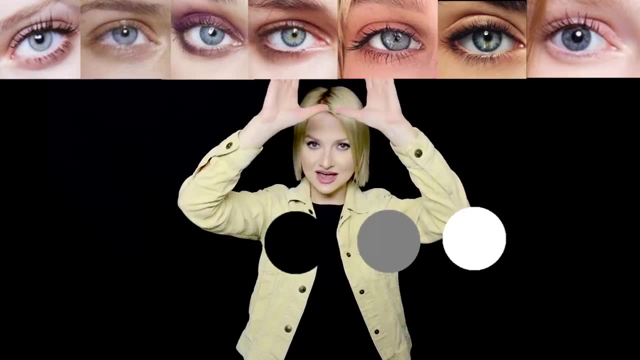 women from lightest to darkest, what eye color they have. so we see that about dark blue color. now if we go to the middle of the scale, this is middle darkness. very often this eyes have some gray color added to that, so it's kind of blueish gray and sometimes 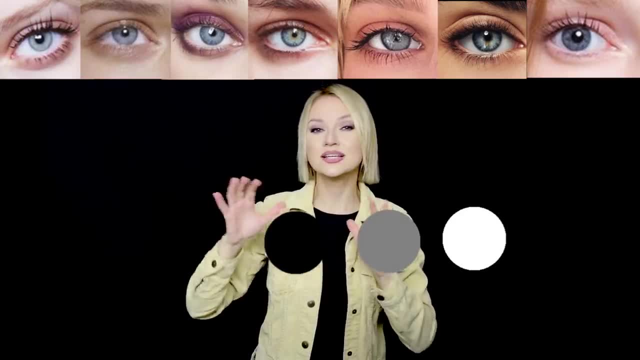 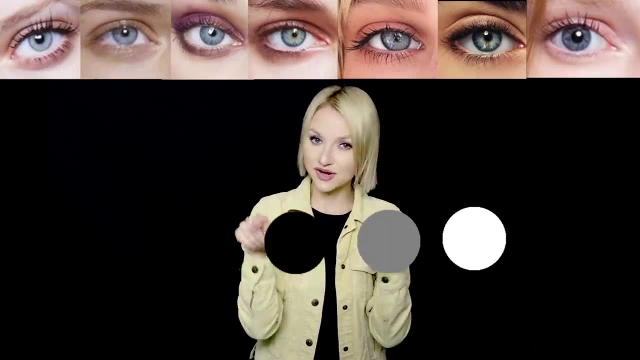 they can look slightly muddy, they can look grayish, slightly dull and less understandable, but they're still blue if you come closer. if they don't have that round circle darker frame and around the iris they can look definitely less contrasted. and if they do have that frame they do look brighter more. 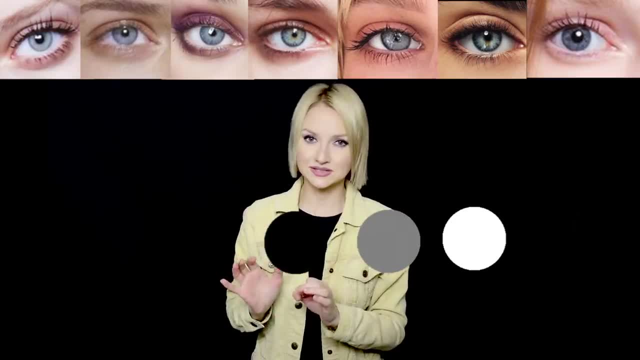 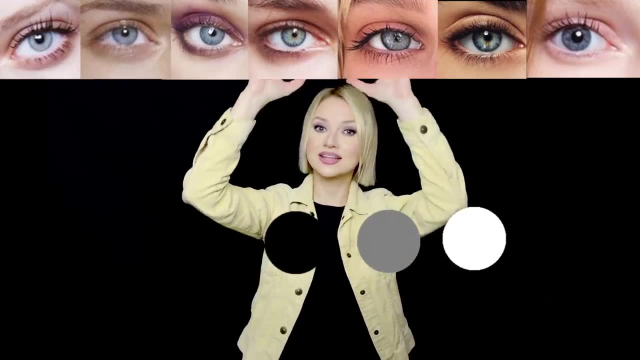 contrasted with the whites and more understandable from the distance. maybe a person with more dull and ashy appearance, more grayish appearance, will have those eyes. However, at the same darkness level we can have another eye which would be very bright: blue, intense color, not the 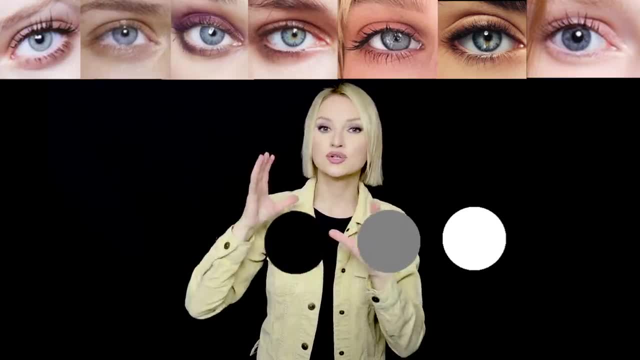 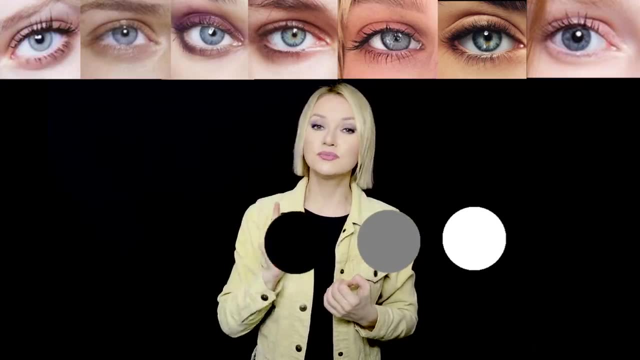 lightest, not the darkest, but still very clear and intense. So normally people with clear complexion, intense, bright complexion, shining complexion, can have those eyes. And again, from the distance this color is pretty simple. Everybody can say, oh, she has blue eyes. So if you go to the lightest shade, sometimes they 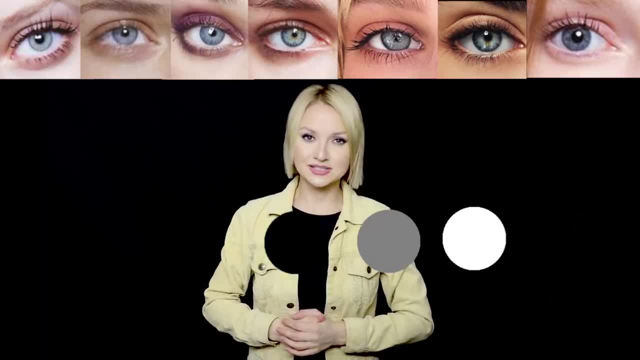 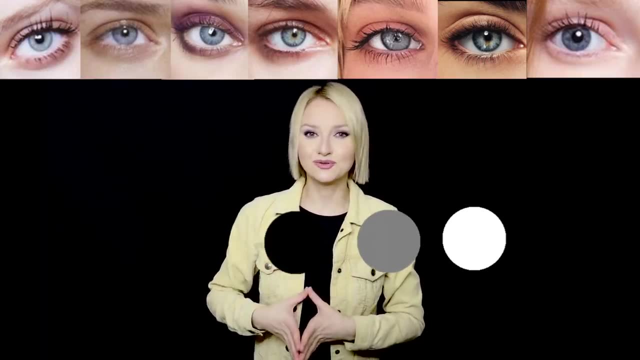 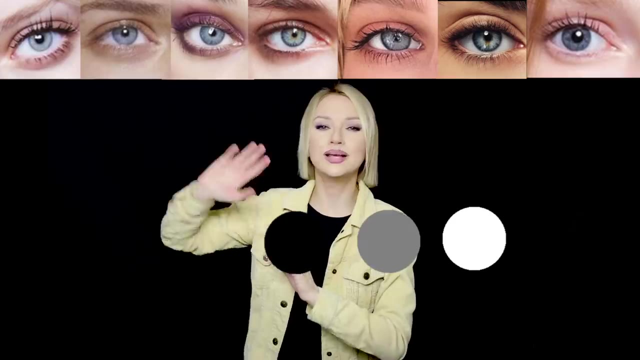 call them silver eyes. Many very light women they have silver eyes. They're not as many people have this very, very, very light and it looks very interesting, very beautiful. So they look slightly transparent and as far as they have a lot of white color, not as much gray color anymore, they have more white color. 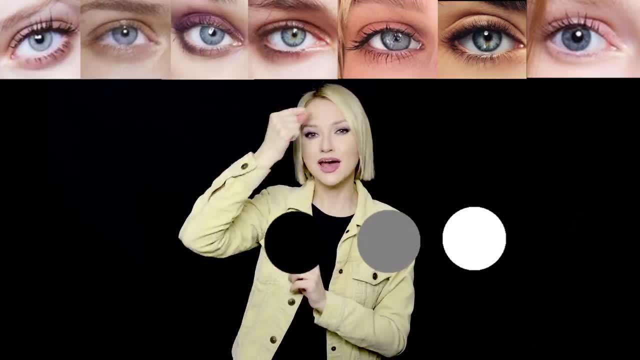 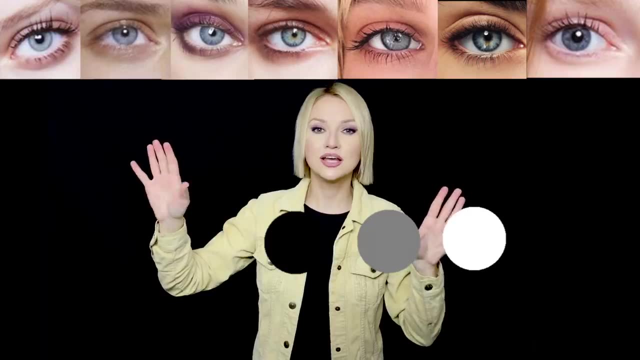 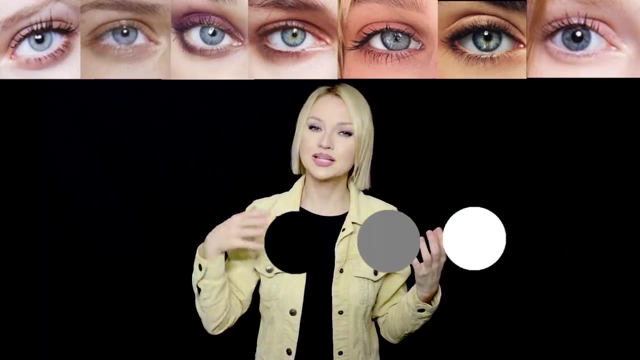 added to them, They look more pale. If they don't have the darker circle around their iris then they look very blended into whites. They look transparent, Light kind of goes inside their head. They look glossy. they look very light, very gentle, but they still 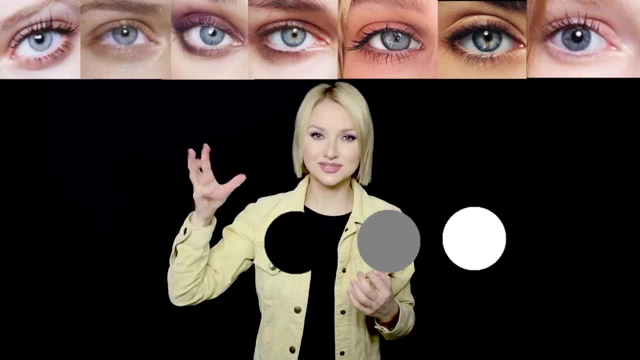 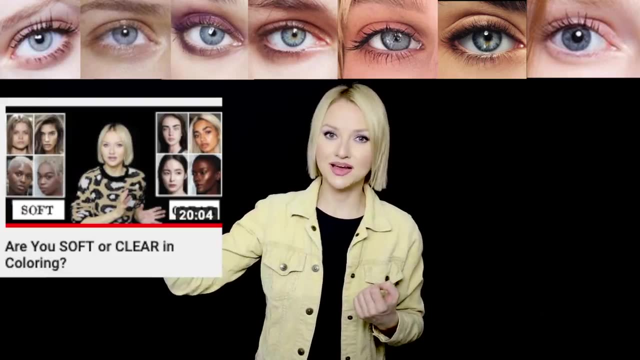 look fresh, They don't look muddy. They have some freshness in them, some brightness and some shine in them. If you've seen my previous video, our Are You Soft or Are You Clear, you will understand what I mean by that Sometimes. 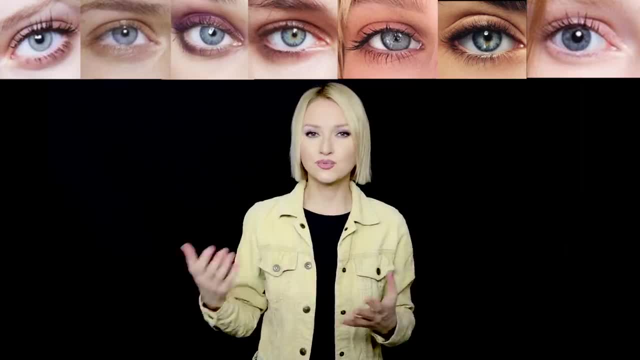 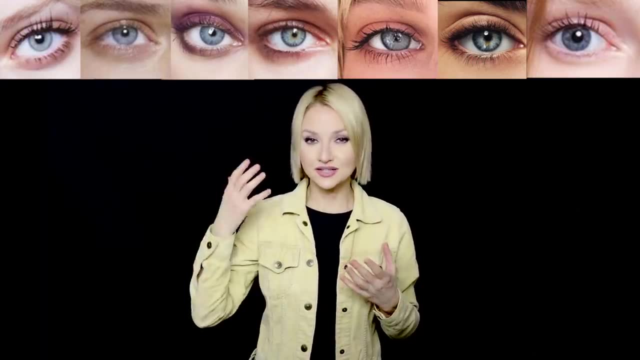 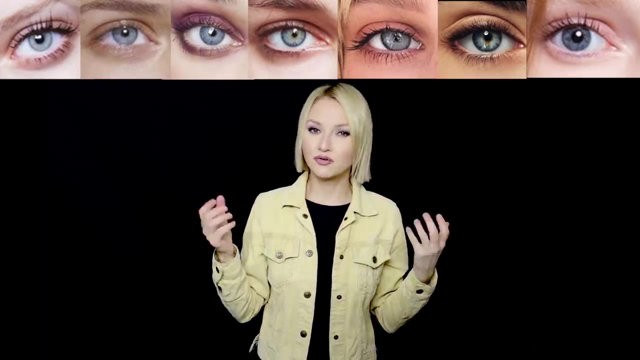 they call them icy blue color. If we talk about coolness or warmness, again, that's an interesting point. Sometimes some specialists, they say that if the person has warmer complexion and he or she has blue eyes, then that blue color is is closer to green color. there's something greenish in that color, but of course most 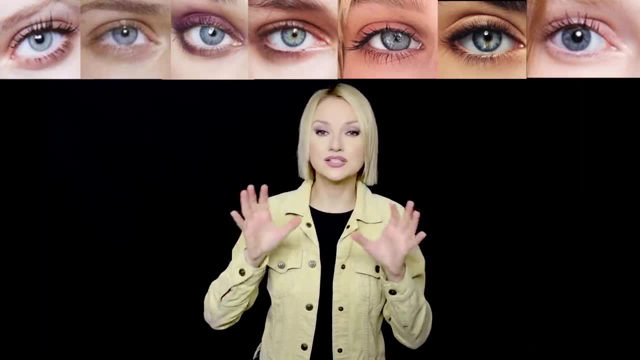 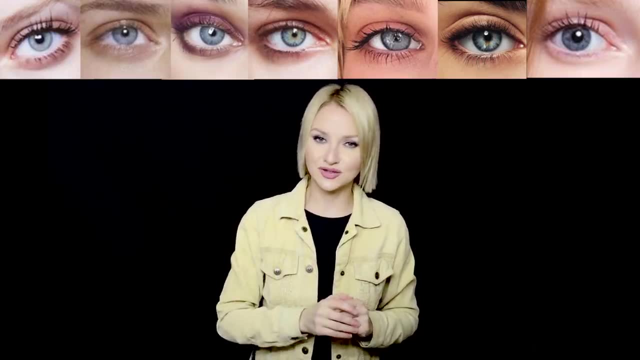 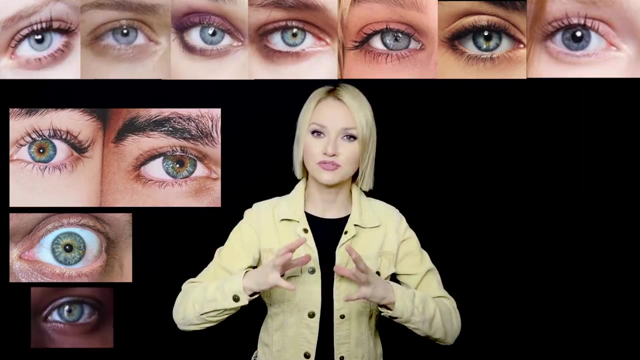 of blue colors, especially if the blue is very clear, bright and understandable from the distance. of course, many of those people have cool undertones. now there are some interesting additions to that. some blue colors can have yellowish circle around their pupil, so that yellowness already gives them some warmth and we don't consider it as pure blue eyes anymore. 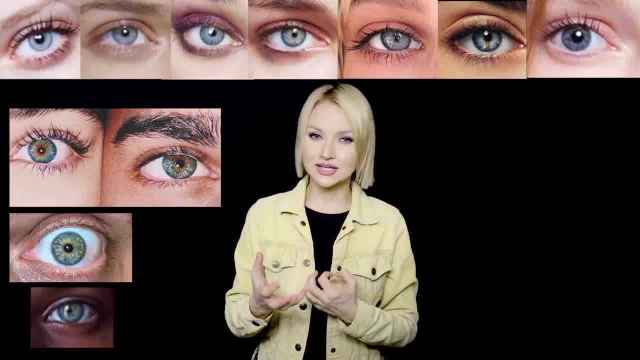 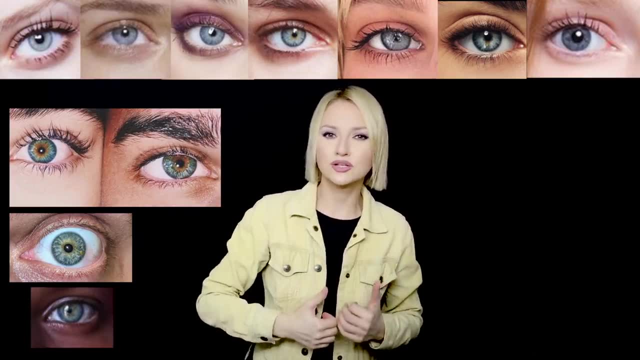 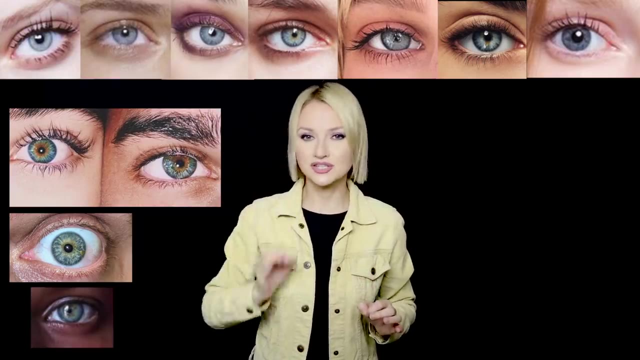 you know, with different light it shows itself differently. it sometimes can look more dull, it can look more muddy. sometimes you don't understand. it can look cooler if he's wearing cooler clothes. can look warmer if he's wearing warmer clothes. they become slightly chameleon because they have some additions to that. that is, making the color slightly more complicated. 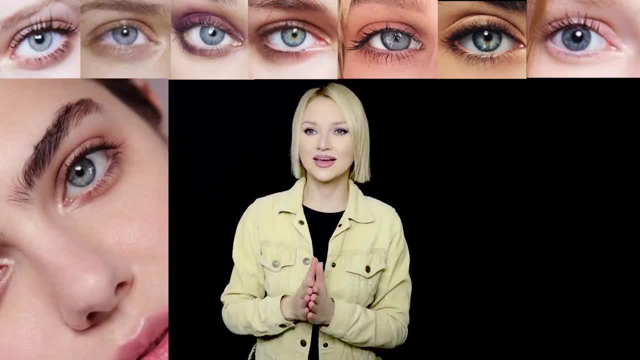 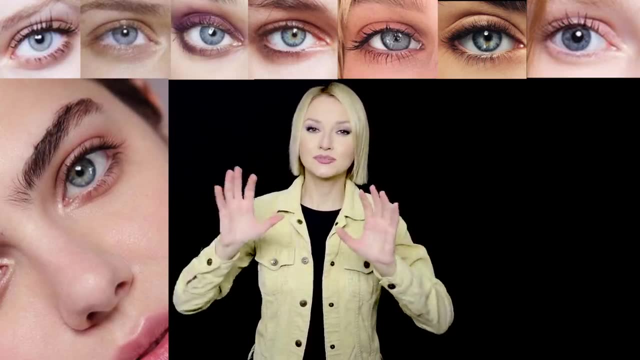 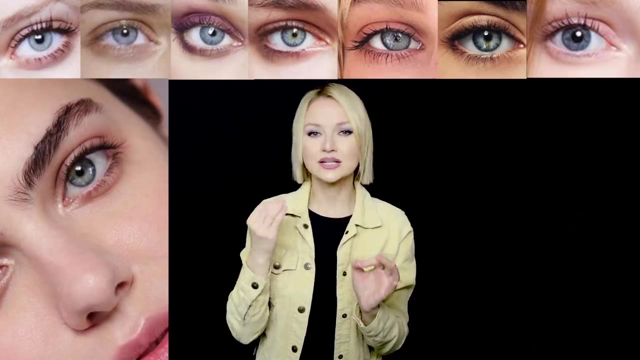 therefore not understandable right there from the distance. and sometimes blue eyes can also be blue gray. they do have some bluishness, but they are slightly dull, as if somebody added some gray color to them. they can be here on the darker side or on a lighter side. they look slightly less bright and less clear in color, less understandable from the distance. and 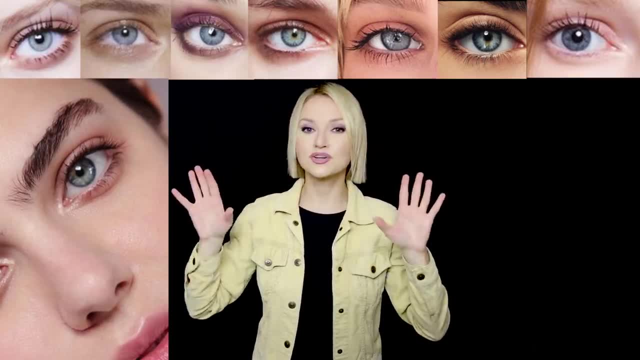 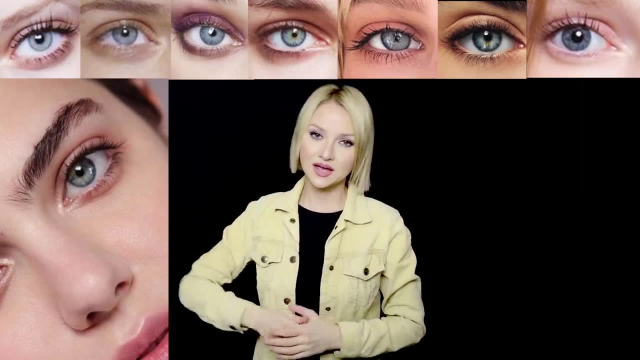 more dusty and it kind of blends with those features of the person and very often this person has slight dustiness on their skin, unless it's very white or slight ashenness in their hair. it just tells us about that. this person has some ashenness and dustiness in her coloration, so she 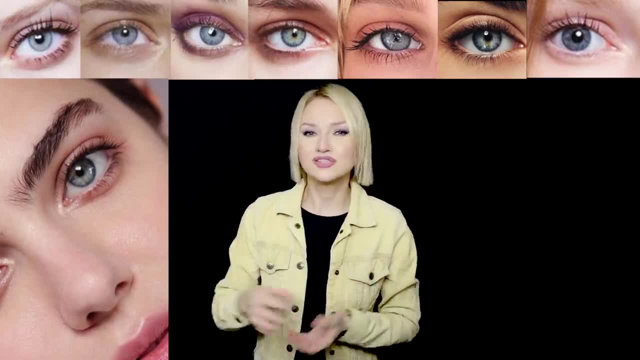 might be able to wear dusty colors a bit more than they usually do, and that's why it's so important to have a dark color on your skin, because if you don't have a dark color on your skin, you can look a little bit more than super bright colors. but again, as i said before, you have to consider. 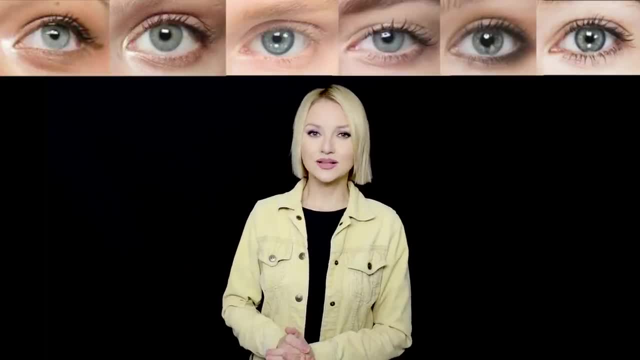 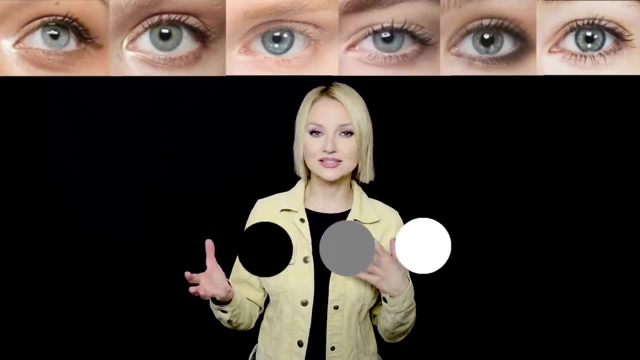 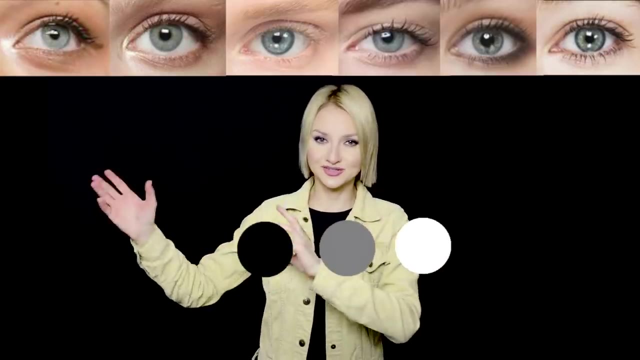 all of the elements. now let's talk about gray color. now, gray color already has gray in it, right, and everything that has gray in it. it looks slightly dull and less reflecting light, less contrasted, less bright and less clear, and gray eyes also can be on a darker side, on a lighter 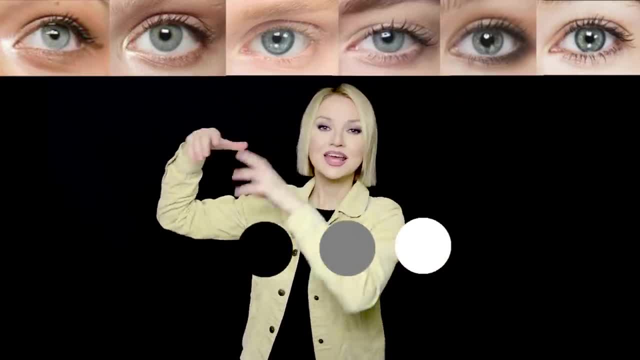 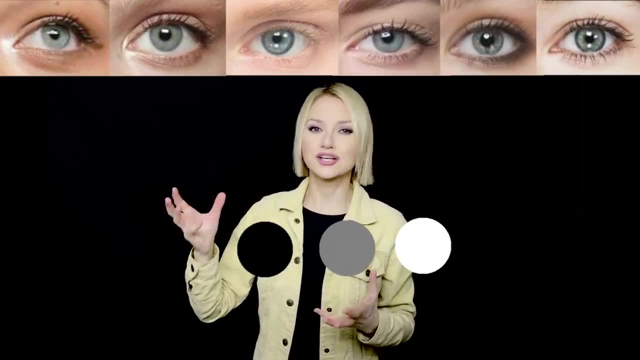 side, like darker gray and then going somewhere in the middle and then lighter gray. light gray eyes contain a lot of white color, so that gray color can be on the darker side. on the lighter side, gray color is pretty fresh still, but it's a little bit harder to name the eye color some people might. 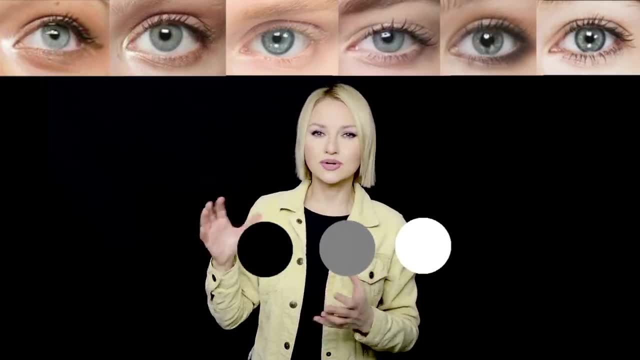 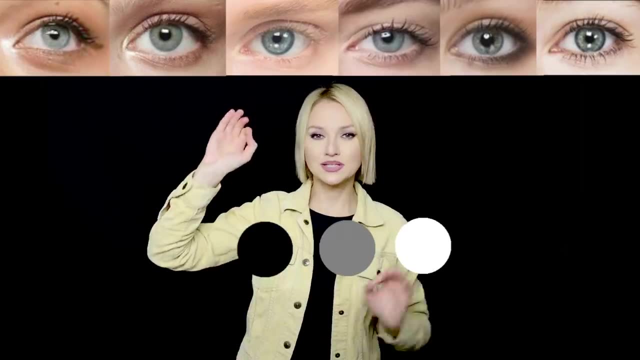 say they're like light blue, light green. so gray color is slightly at that point when you sometimes can't say, and with different lighting it kind of changes its color. it happens because different lighting has its own kind of coloration and also it reflects from the environment. so all those 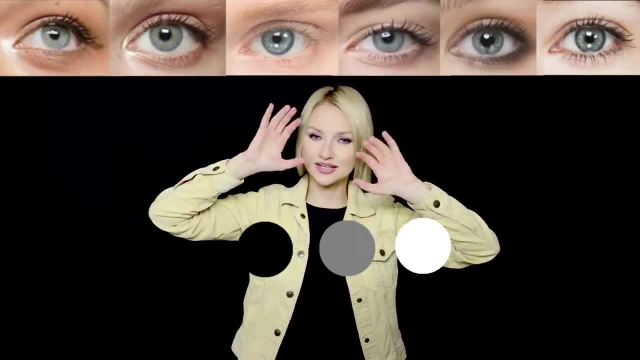 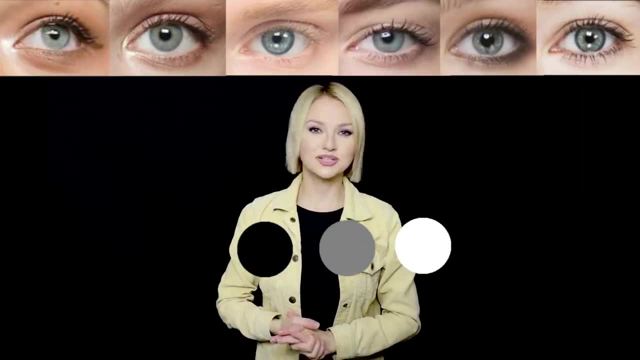 colors kind of go there and kind of mix with that gray color slightly. it gives you sometimes that illusion that it has different colorings and it's a little bit harder to name the eye color. but in general gray color is pretty neutral color and it's pretty dull and slightly muted and ashy. 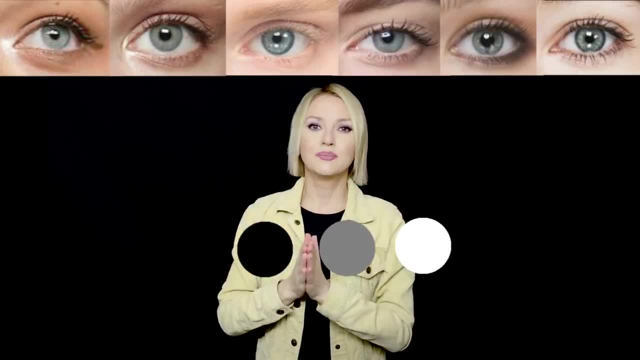 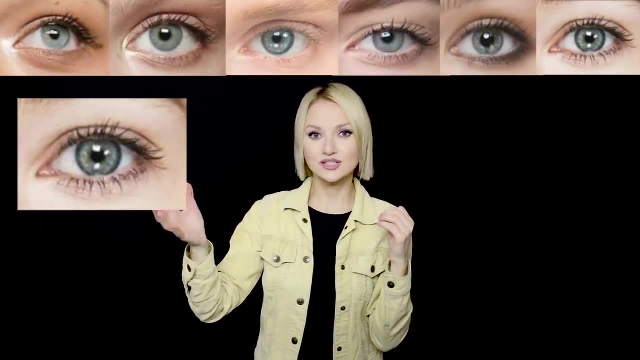 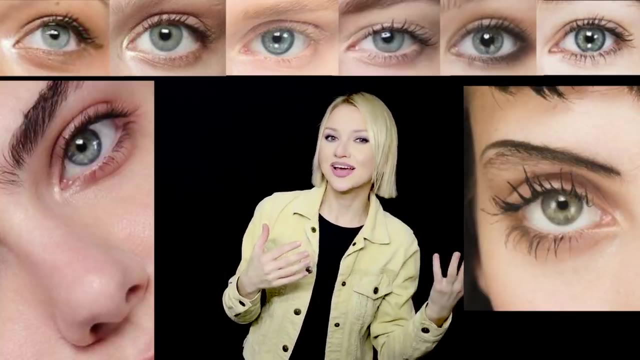 so many people who have pretty ashy hair, for example. they can have gray eyes. gray eyes again. they can have this frame. they will look more contrasted and slightly darker, or they might not have this frame. some may be on a bluer side, some on a grayer side, on a greener side, some can. 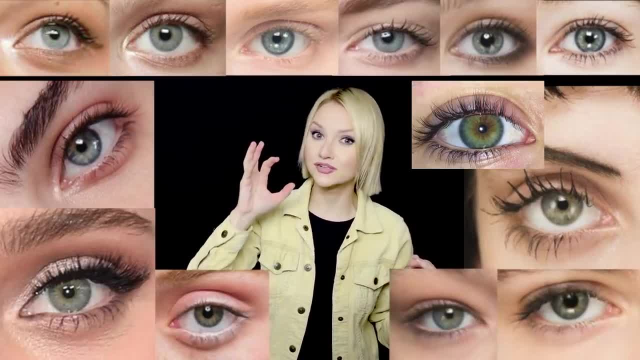 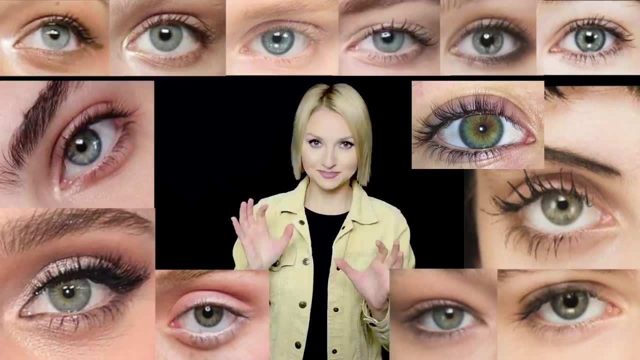 have some additional colors around the pupil, some greener colors around the pupil or, yeah, yellowish colors around the pupil, it will look like muddy, warmer gray color. but in this case, if you do have some, let's say, yellowish coloration around your pupil, you have to see how much of the 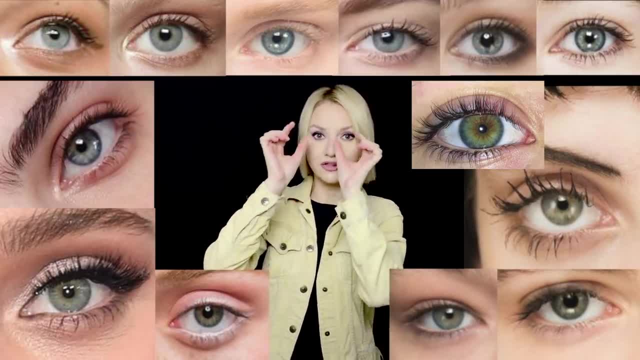 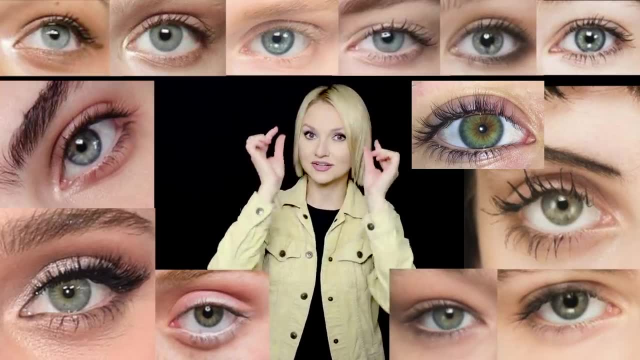 space of your iris it takes. so some people they have a lot of that color and their frame is different color. let's say they have a lot of yellow color but their frame is dark gray or dark blue color. that gives that more complicated color. but the more yellow color there is, the more on a 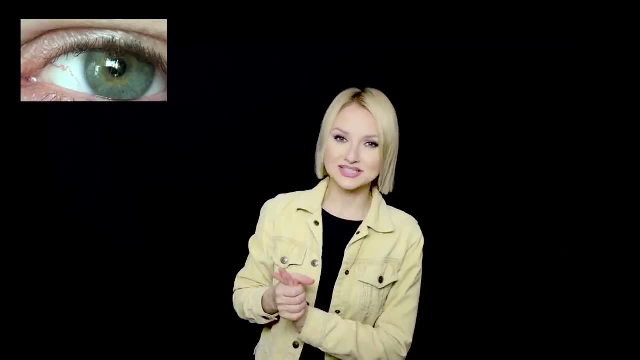 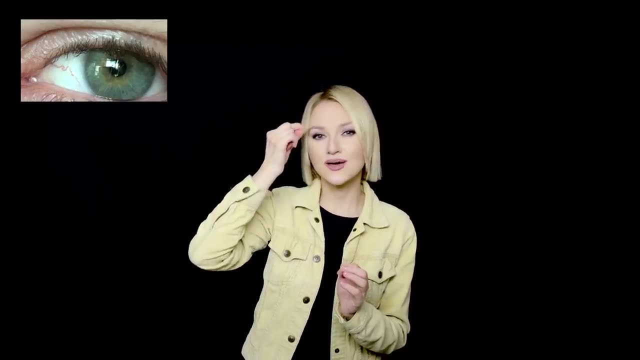 warmer side, the person will look more yellowish and the more yellowish color the person will look. we did some experiments with my husband's eyes. his eyes are pretty light. they're not very clear. the color is pretty complicated. he has some yellow circle around his pupils and then he 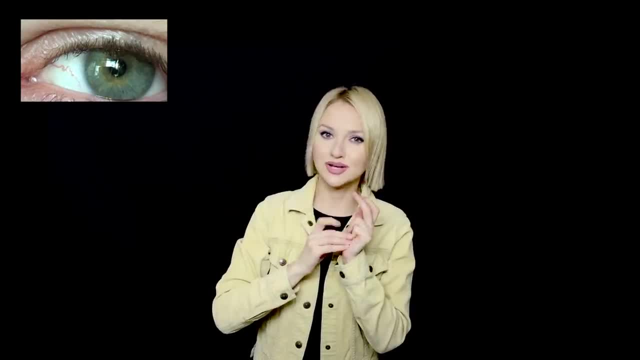 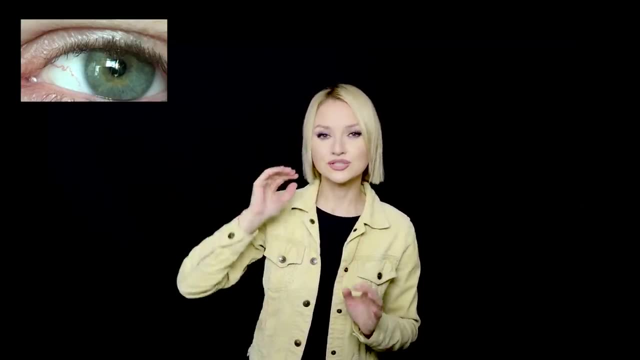 has some interesting color. sometimes it looks green, sometimes gray, sometimes blue. it depends on the lighting, where he is and what he's wearing, and we put some of his T-shirts close to his eyes and we started comparing them to them when we put light blue color to them. 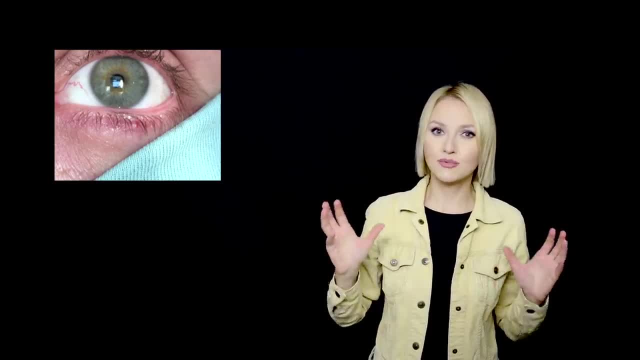 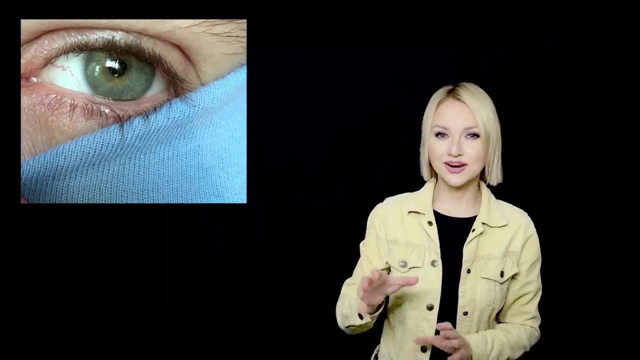 we could immediately see that his eyes look more dull, more muddy, more gray, not as fresh, not as clear blue, not as transparent and glassy. If we put darker blue, but still very clear blue and very cool color, we could see that pretty much same. 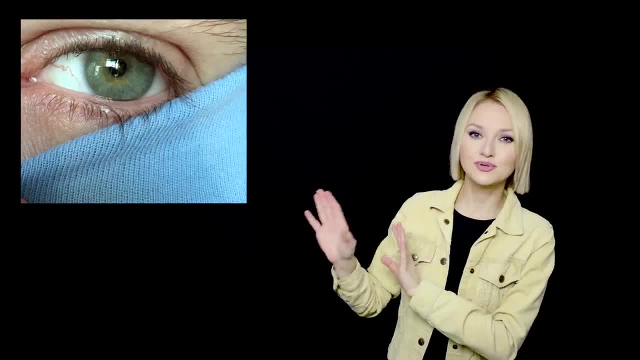 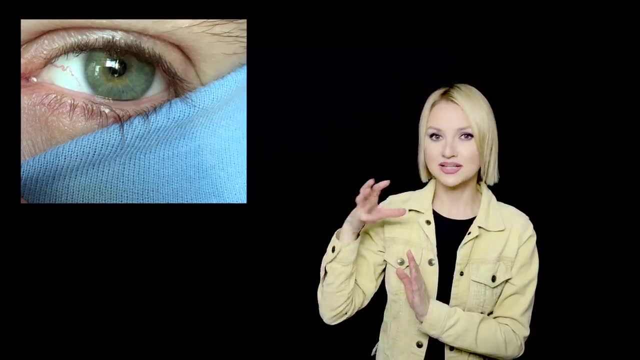 darkness, but his eyes look warmer with that because that is pure cool color and his eyes have some yellowishness around his pupils. so you can see how warmer they look, but they still look slightly muddy and slightly dull. Again, not as understandable color, not as clear. Then we tried. 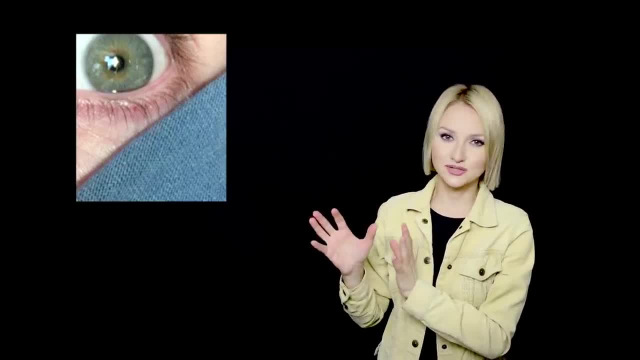 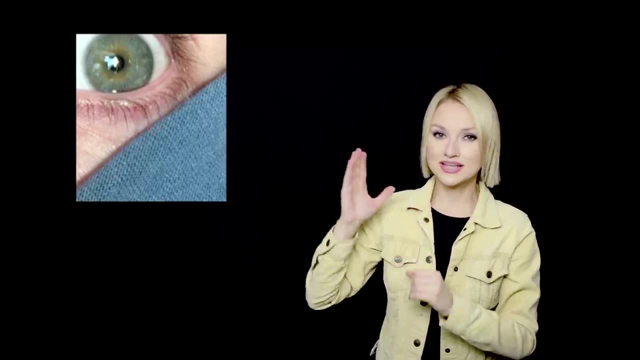 darker blue color- still pretty cool color, but with added gray to it. So now the t-shirt color is darker, his eyes are slightly lighter, but the dullness is still same. but again the t-shirt looks cooler and his eyes look slightly warmer just because of that. And then we finally found that 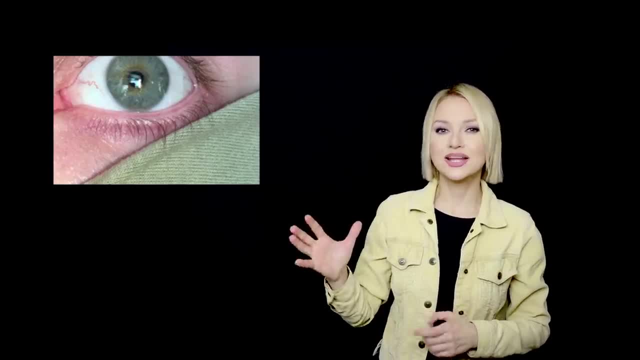 green hacky color t-shirt that is on a warmer side but has a lot of gray to it and it's somewhere in the middle of darkness and lightness. So it's not dark, not light. has a lot of gray dullness to it. 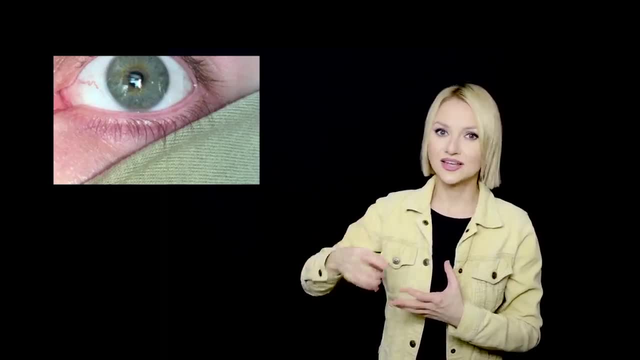 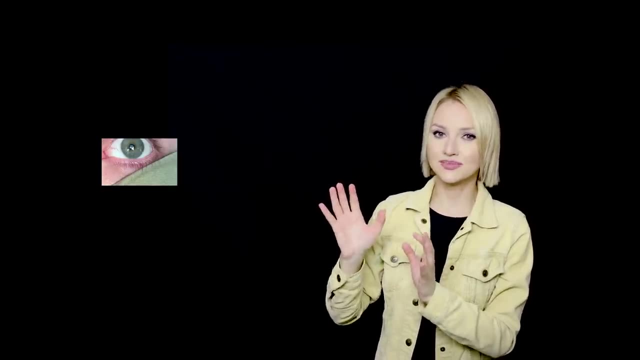 like ashiness to it. not clear, bright green color, Like grass green right, And it matches it pretty much matches. From the distance we could see it is approximately same color. If you look closer, just on his eye, you could see blue in it. 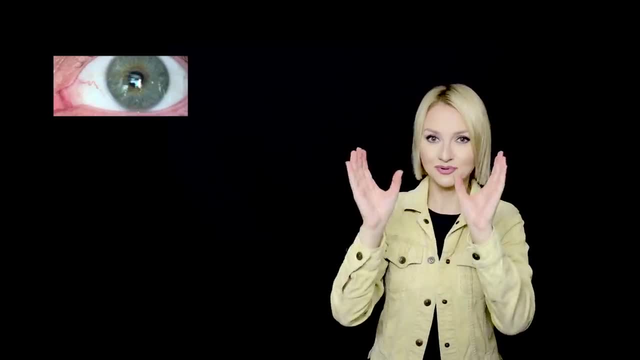 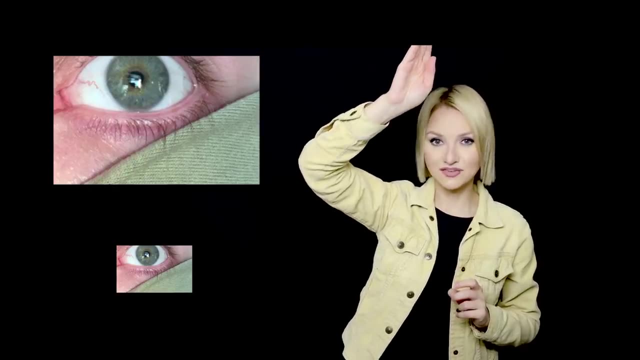 and yellow in it. They are not mixed together, they are like separate. but from the distance it mixes up and it matches In the scale of the darkness and lightness. his eyes are somewhere in the middle, not very dark, not very light, maybe slightly to a lighter side if you compare. 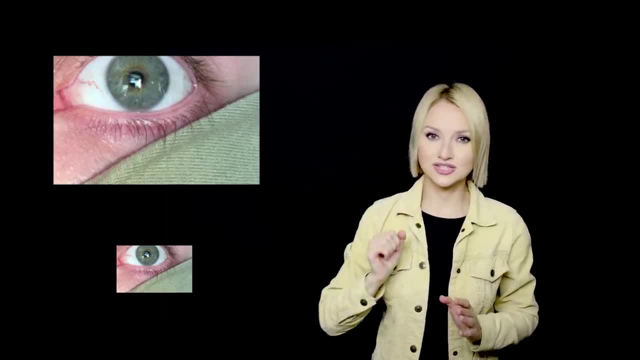 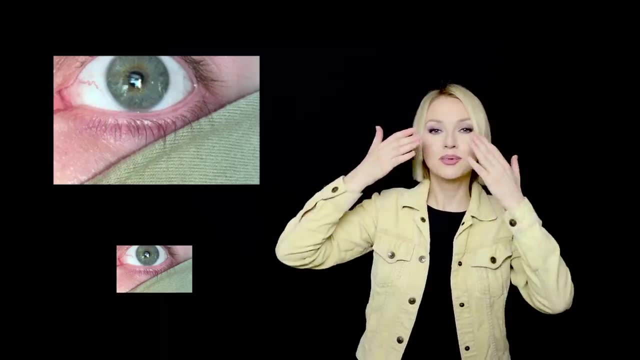 him to other people, let's say, And it's muddy and not contrasted and the frame around his iris is not very bright contrasted and not very dark. This way, from the distance, it kind of blends into his whites a little bit. Now, green eyes. About green eyes, I heard that 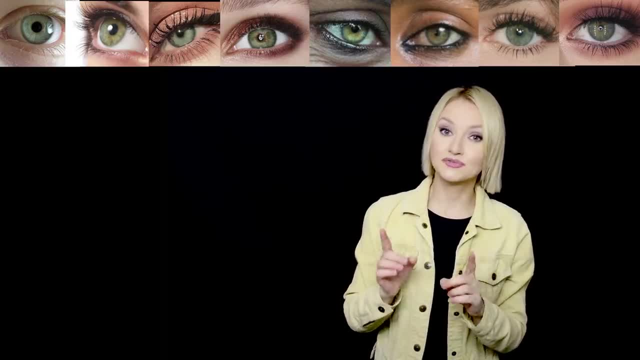 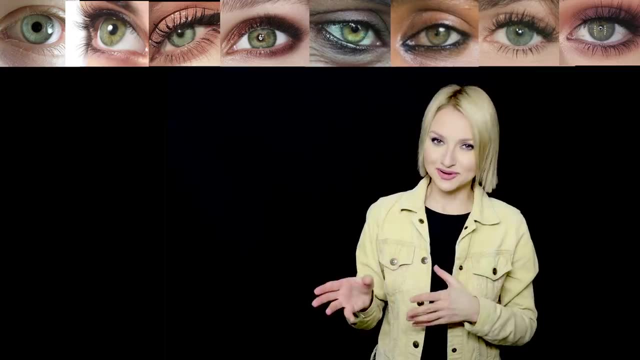 only 2% of people have green eyes and 80% of women and 20% of men have it. It's more a female color of the eyes. it's interesting, And most of them live in Europe- in Hungary and in Ireland, And 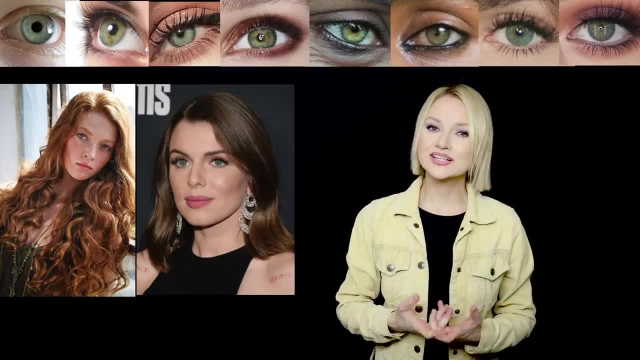 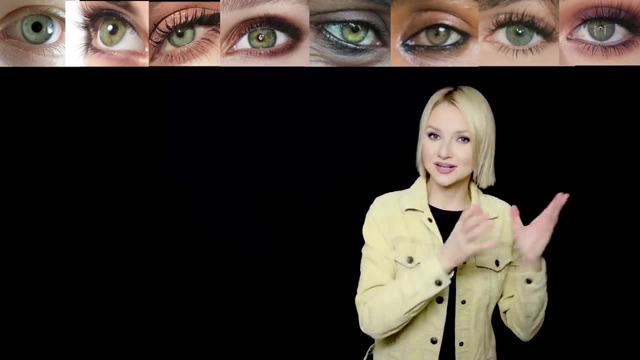 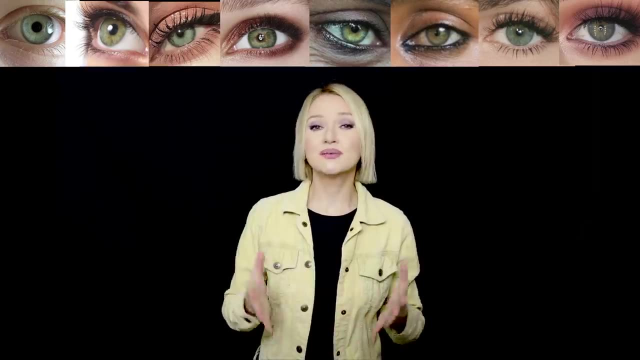 many of them have red or reddish hair. Normally it stands for warmer undertone, but in this case it's more of a warm undertone. And again, green eyes can be on a darker or on a lighter side, And also there can be some additions to green color. It's not as clear Sometimes it can be. 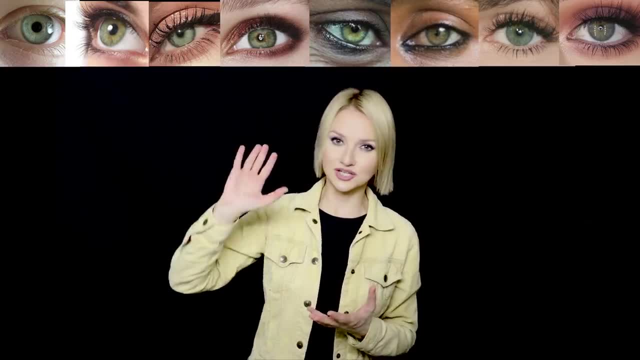 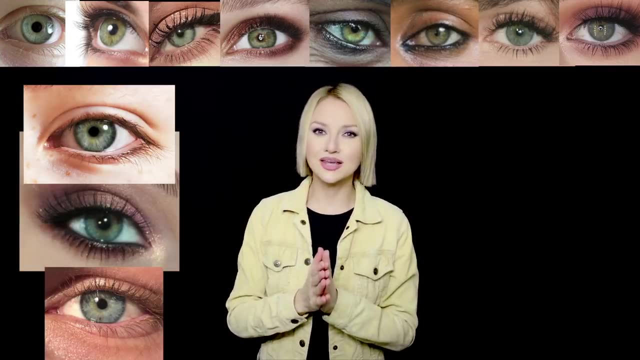 very clear green color on the eyes, no matter on which lighting she is. Sometimes green eyes can be very complicated. If green eyes have some mixture with blue eyes, then they become slightly on the cooler side, but still not very completely cool. very, very cool. Sometimes they on contrary. 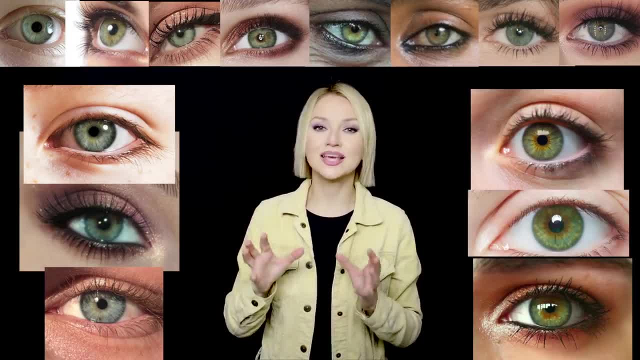 they can have some yellowness around the eyes and sometimes they can be a little bit more on the darker side, but still not very, completely cool, very, very cool. So in this case that green becomes much yellower, much warmer color. Same thing with the frame or without frame. 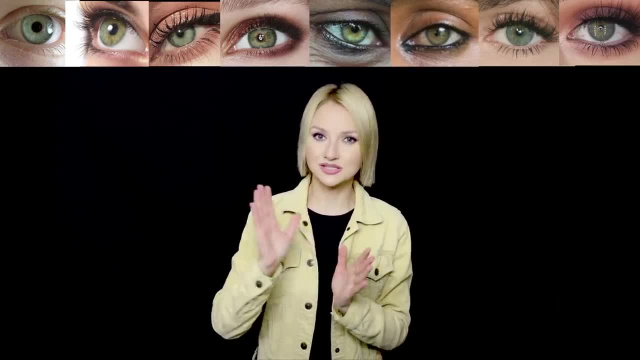 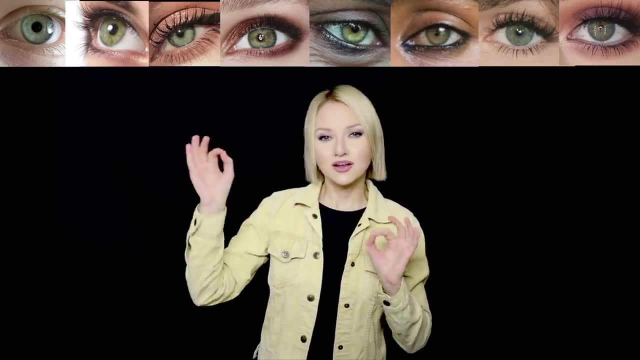 So when the person has very clear green eyes that we can see from the distance that they are green, normally she has pretty clear coloration. If the green eyes have a lot of grayishness to it and a lot of additional colors to it, it looks more complicated, it looks more muddy sometimes. 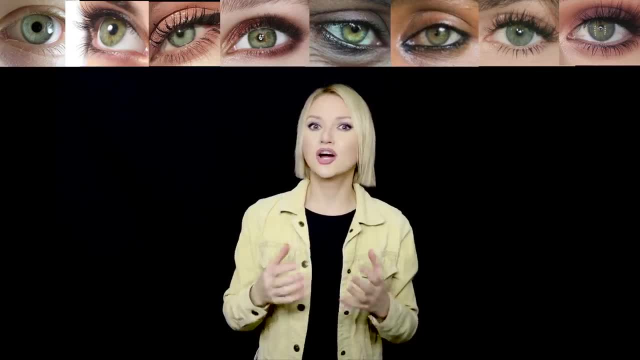 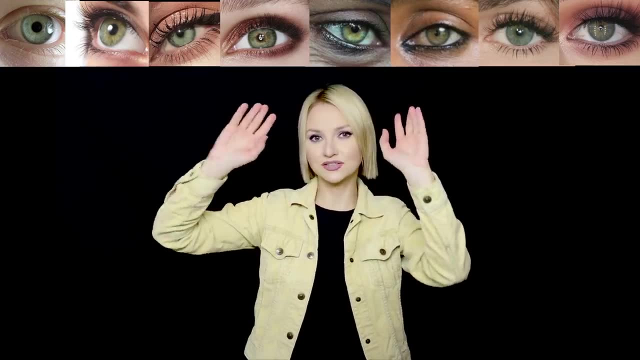 and less contrasted. I haven't seen as many dark, dark, green eyes. I can say that the green color itself it's pretty light color. So we would go somewhere from the middle to the light, and again not to the lightest, not to the very lightest. So I would say that middle area of middle darkness. 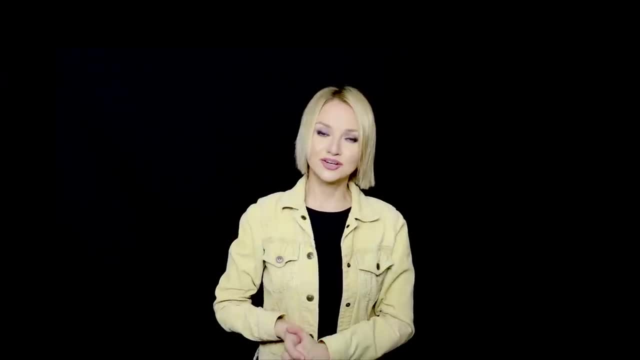 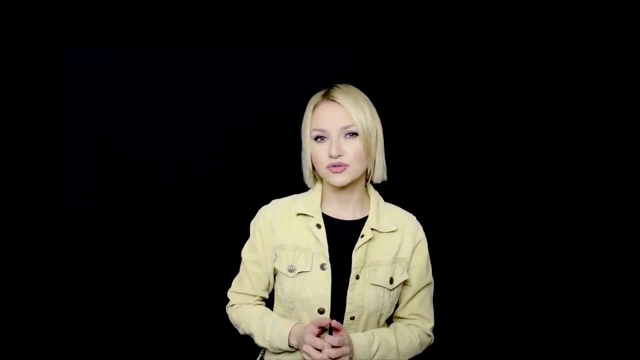 I think this is where most green eyes present. Now, did you know that there can be violet eyes? As I understand, that color really exists. Let me know, guys in the comments, if you ever saw a person with really violet eyes. There was one famous person who had that color of the eyes. 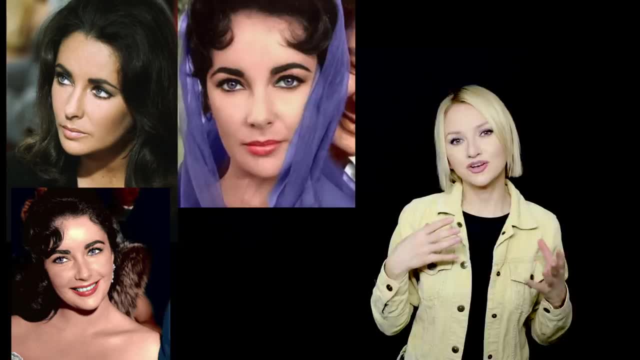 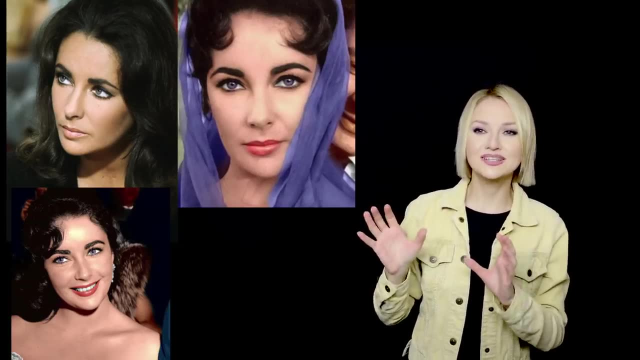 and it was Elizabeth Taylor. At that time photo cameras were not this good so they couldn't show real colors in the person. but I found some pictures that you can really see. you know, and sometimes you can say, oh, it could be added with Photoshop and stuff. but I found several of. 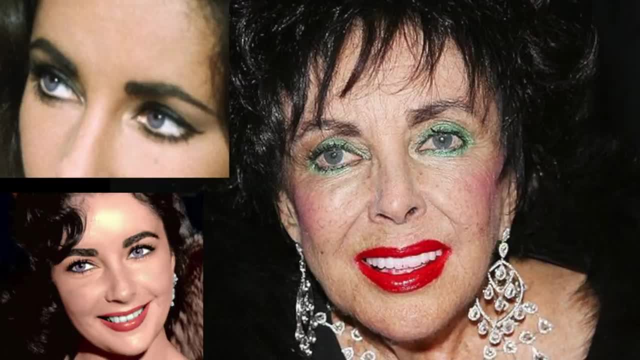 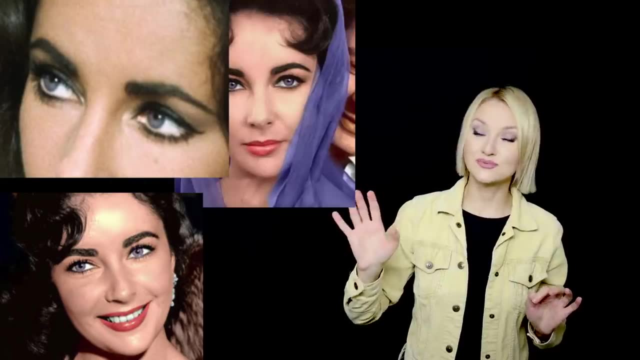 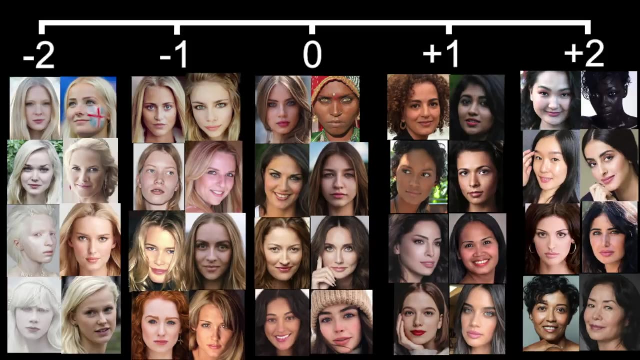 them and you can see slightly that violet color in those eyes. It's very, very interesting. It's very interesting eye color. I would really want to see that in person. Now let's look examples of women from minus two contrast: very lightest girls to the darkest. 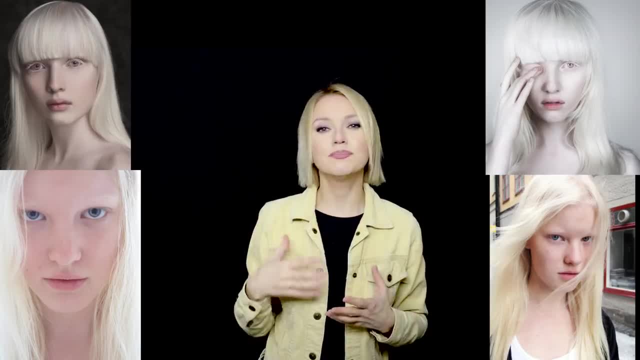 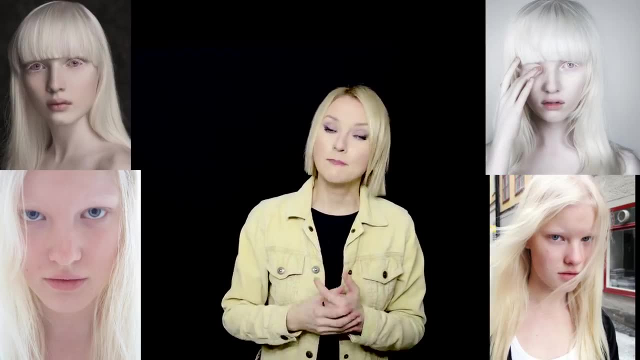 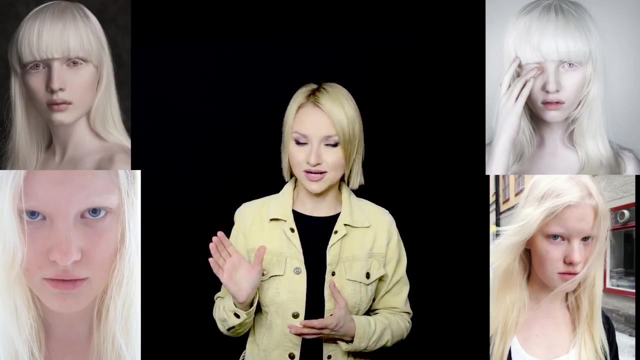 And very bright women. I checked many pictures of very pale girls from albino: very light, pale women with white skin, very light hair. Most of them have light eyes, of course, light gray or light blue, But first I thought that I would only see very light blue eyes, which is not the case. 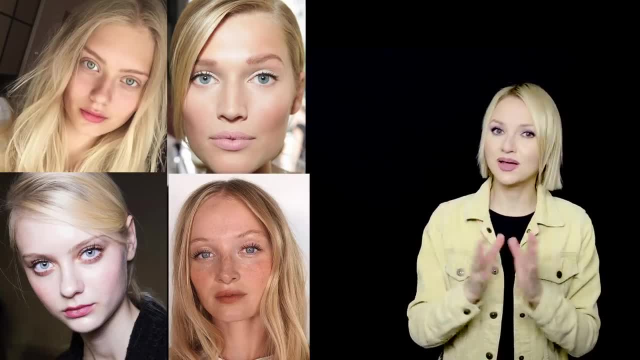 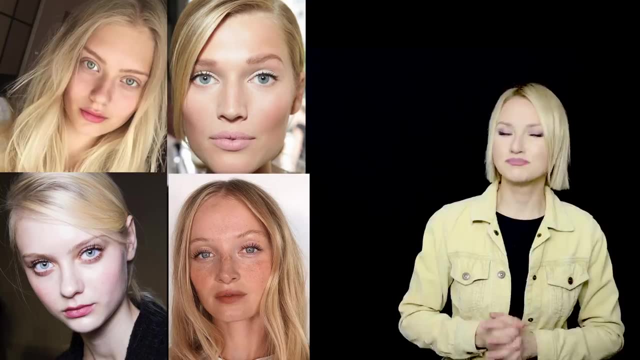 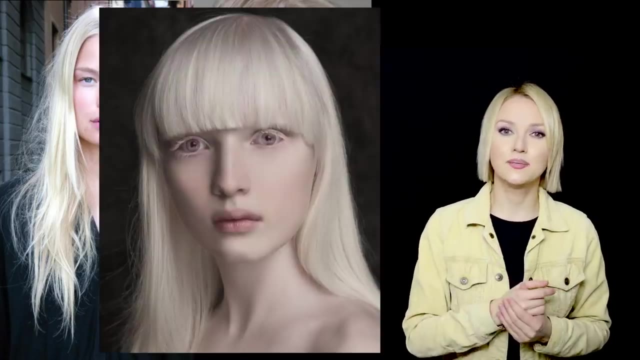 Many of them have darker blue eyes actually and many of them have kind of blue-gray eyes and their eyes are actually slightly more contrasted than the rest of their appearance. Light green color- rarer, But still can be the case Normally. yeah, very silver light eyes and slightly darker And 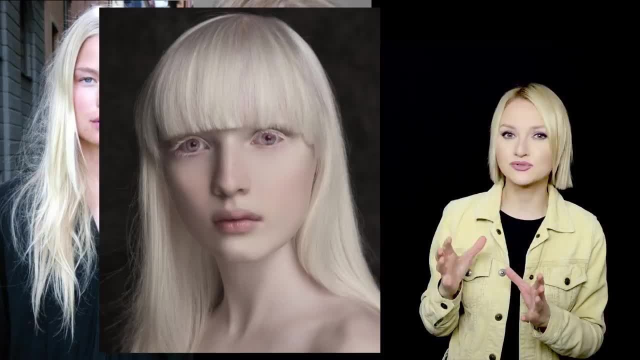 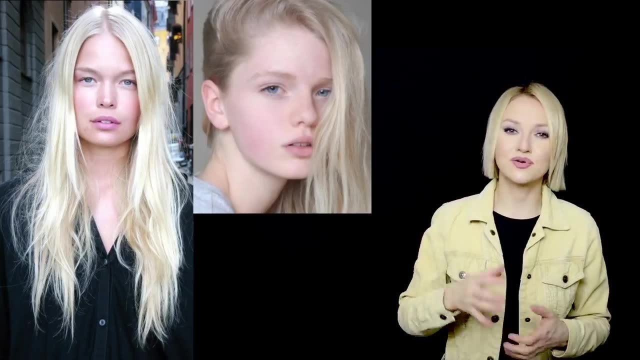 albinos. actually they can have some reddishness in their eyes, which is also very interesting. Most of these girls with that very light blue eyes. they have a lot of white color added to them so they have very fresh palette of colors, light and fresh appearance. And those with darker. 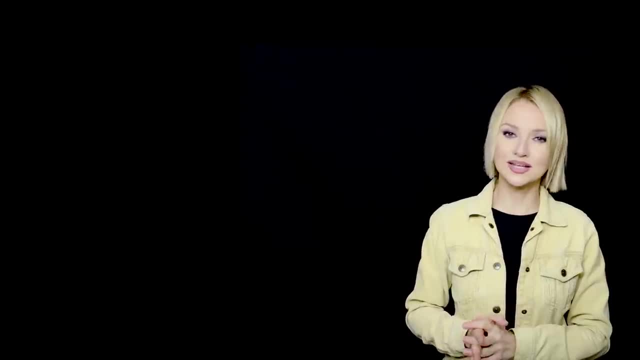 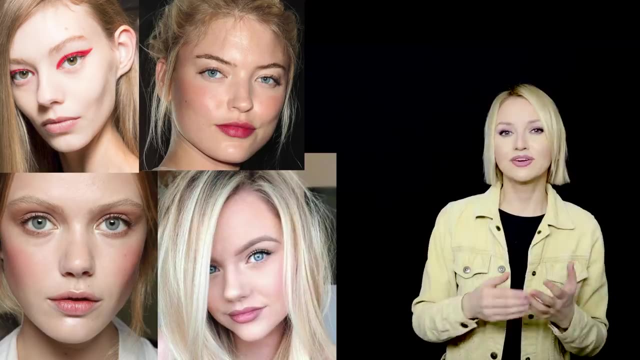 blue eyes. they can have slightly more contrast, Minus one. In this category women already have some color added to them. They're not as white anymore. So in this category we also have a lot of light. gray eyes, blue eyes, but also in this category. 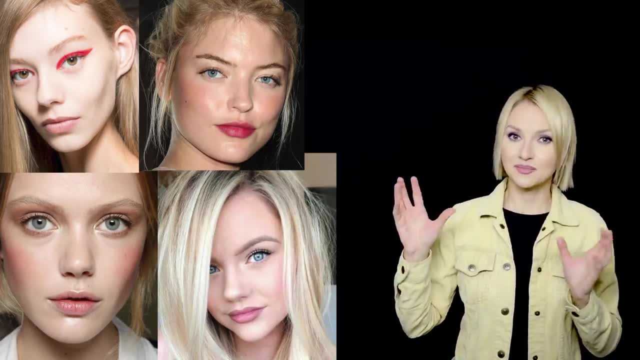 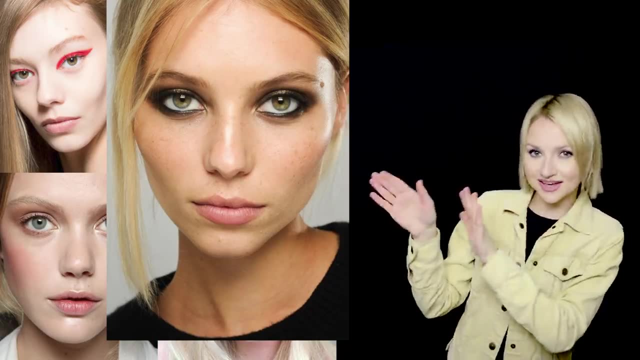 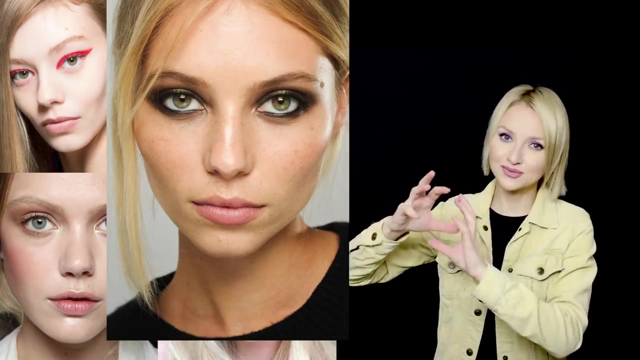 we start having those yellow eyes, amber eyes and some hazel eyes, light hazel eyes. This is the attempt of those darker brown colors to kind of sneak into that category, So it kind of reminds about itself a little bit on those colorations, But still there's a lot of white color added to. 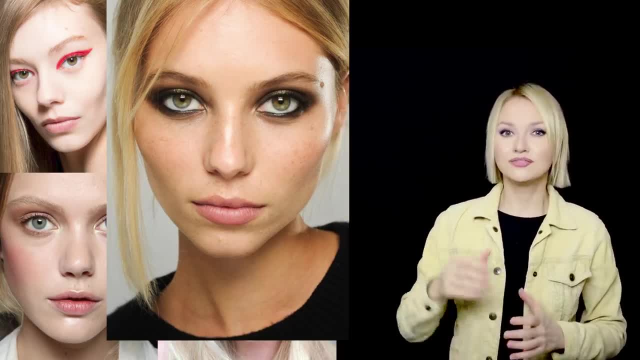 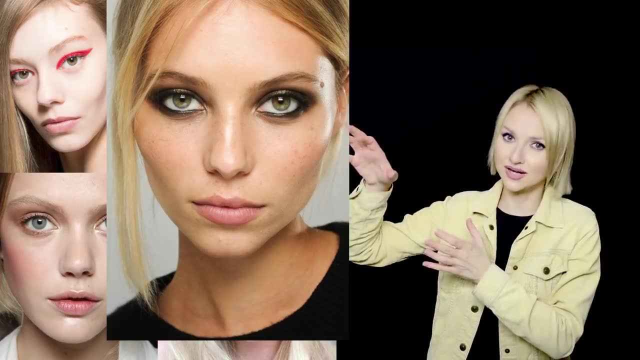 that. so it's pretty light on the lighter side. So if there's light, hazel eyes, probably that's what you're looking for. But if you're looking for a slightly muddy, slightly, with some additions of gray color to that already, so they can be slightly muted, not as fresh looking, not as clear. 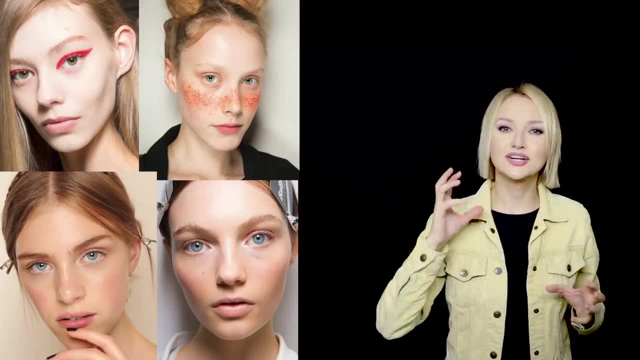 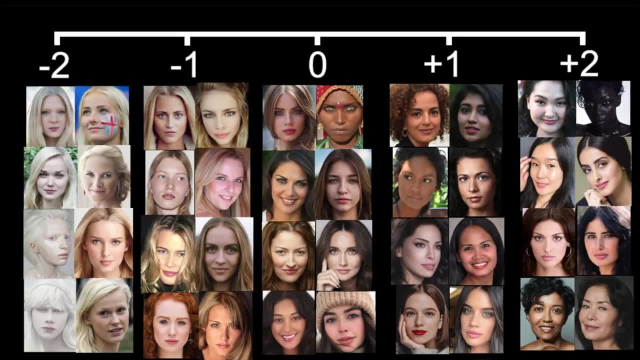 and bright looking And, of course, if they have their clear blue eyes, clear amber eyes, then they have that more clear appearance about them. Zero contrast, Zero contrast on the scale of darkness and lightness. They're in the middle, so they have a lot of gray colors presented in them. 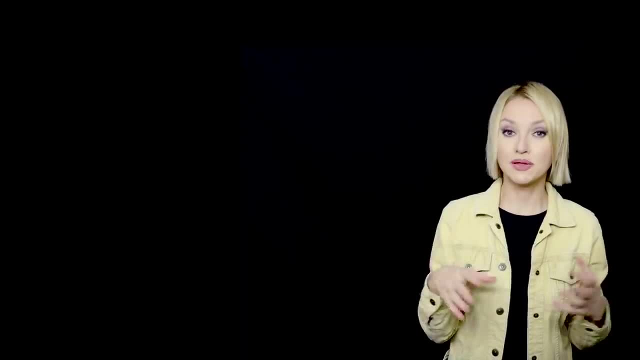 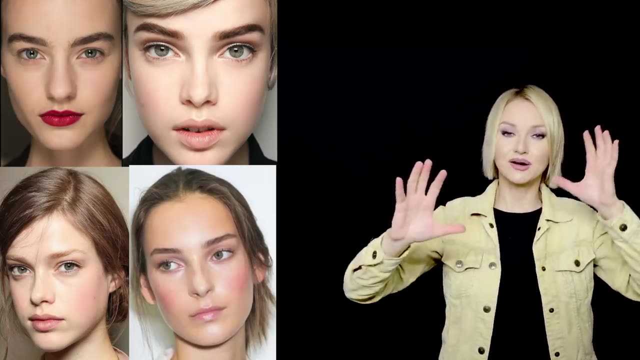 They're not as light anymore, so they probably have some darker colors in them, But they're not as dark still. Their complexion is still reflecting light pretty good, so they are somewhere in the area of very dusty appearance, very dull and muddy appearance. 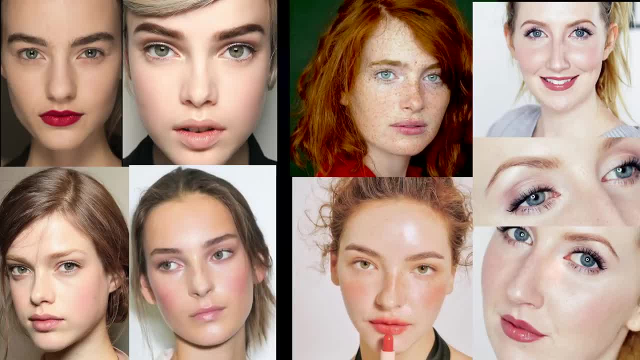 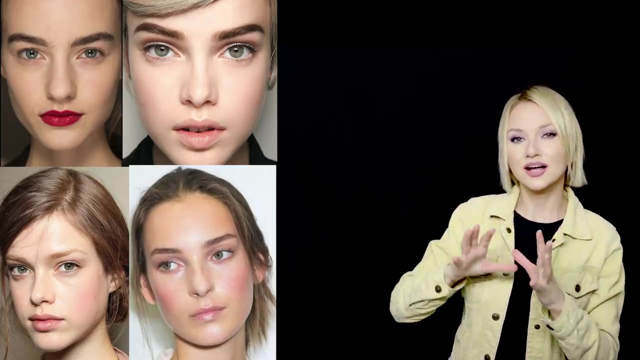 or, on contrary, very bright. Let's say she has orange hair, light red hair, Normally redheads in this category. they have pretty clear blue eyes or clear green eyes and sometimes very clear brown eyes on the lighter side, And girls with muddier complexion with more dull and more. 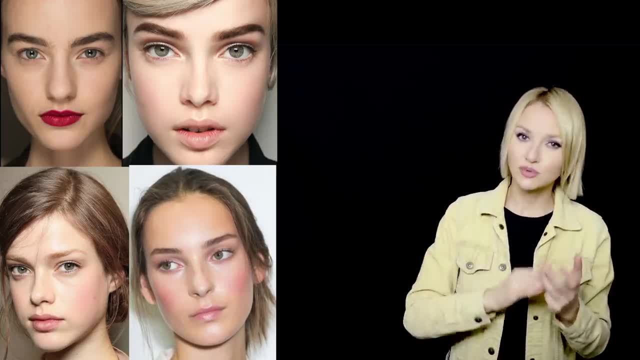 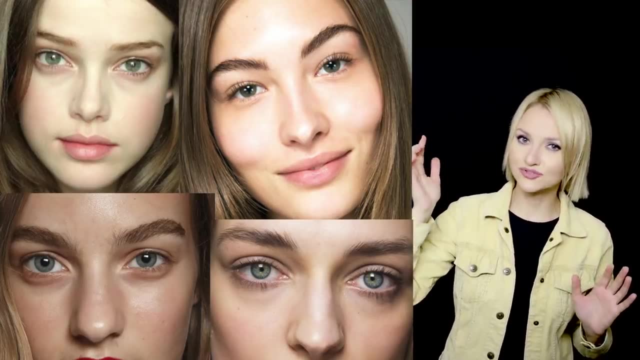 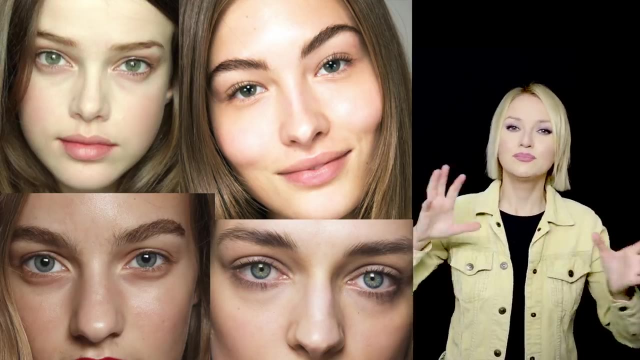 soft complexion, more muted complexion. they can have those complicated eye colors that I told you about, Some complicated colors, some additional rings around the pupils. They can have some yellow plus dark, gray, yellow plus green, yellow plus brown, brown plus gray. All those. 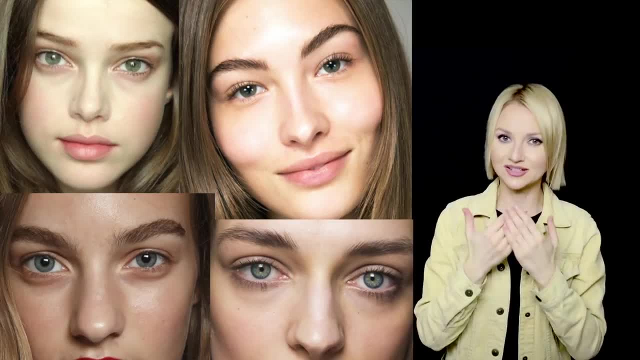 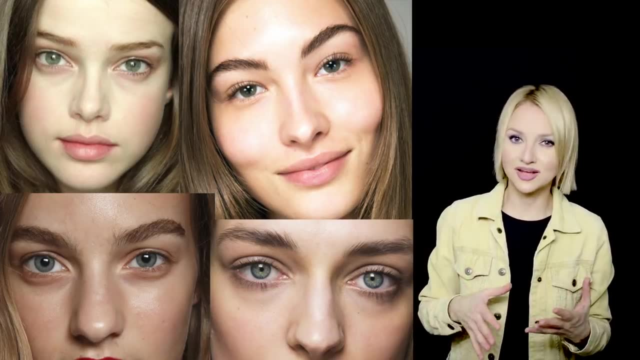 contradictional colors that just clash in their eyes. you know They also pretty often blend into their whites. We can't see the eyes right away, so they can have soft brown eyes or soft blue eyes, And in this case soft blue eyes meaning blue with added colors to them. 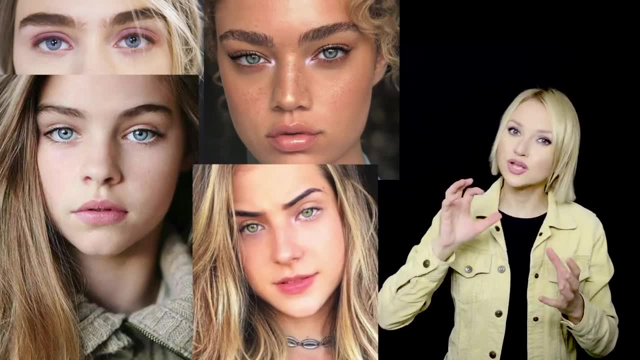 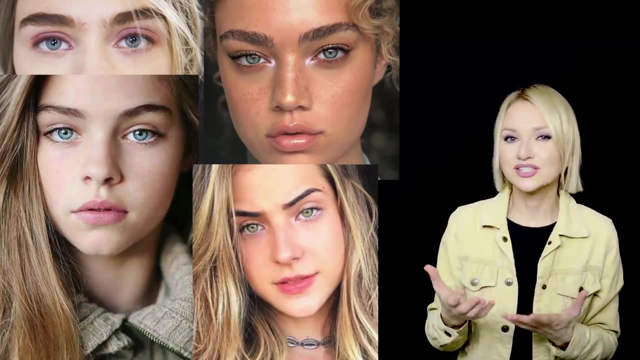 blue with added gray, darkness, grayishness to it. blue with added some green tones to it, maybe some brown tones to it. This is sometimes why it's very hard for us to say if she's on a cooler side or if she's on a warmer side. She has kind of both of those colors exist in her. 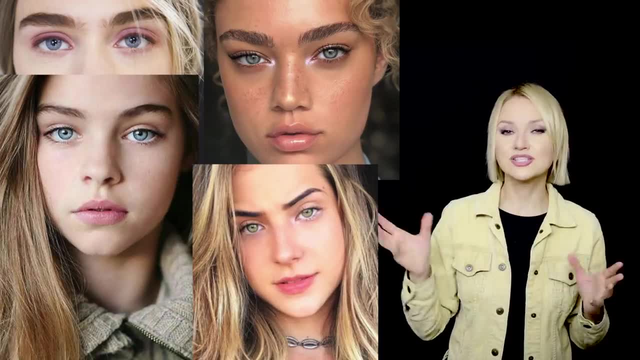 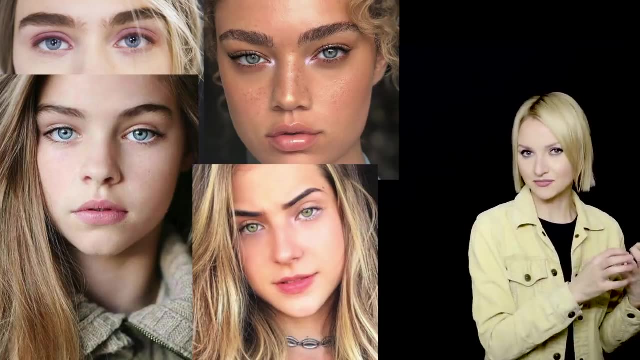 appearance If she consists of more brown colors, let's say, but she still has a lot of gray to it which kind of dulls that warmness a little bit And it kind of brings it slightly to a cooler side right. In plus one contrast category. 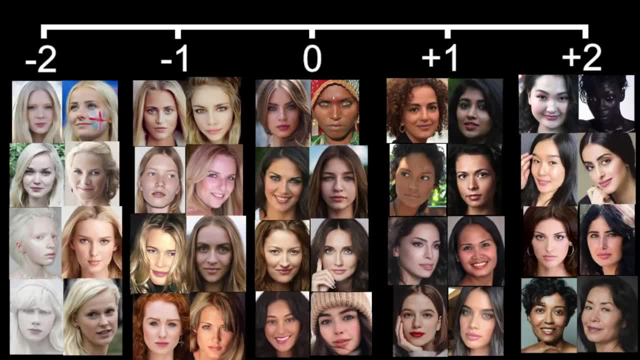 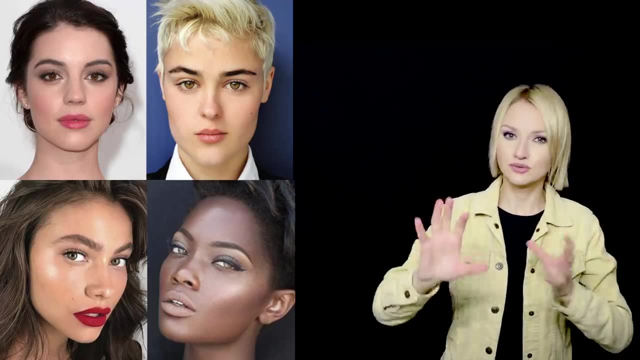 we already have those reddish brown colors, intense brown colors, Maybe not black. Black is still so contrasted with white, so probably goes to plus two contrast category. Here we still have some reflecting of the light. In plus one category, women have gray and black already added. 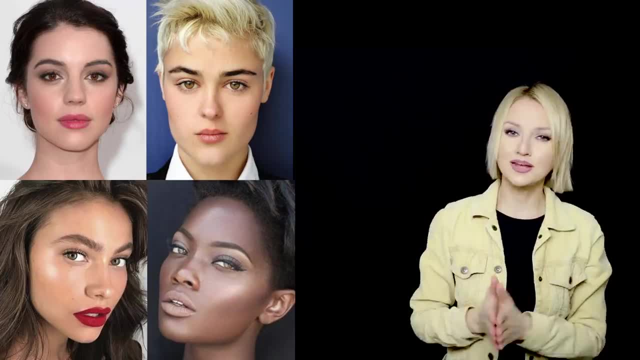 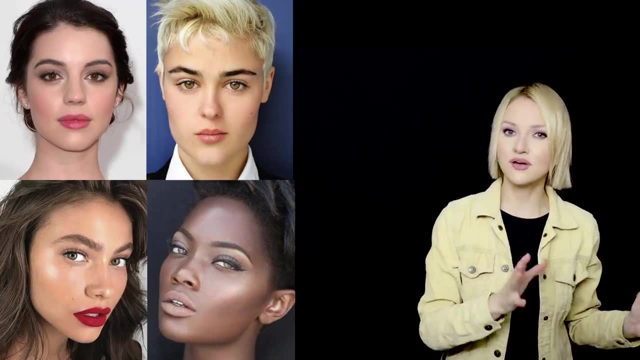 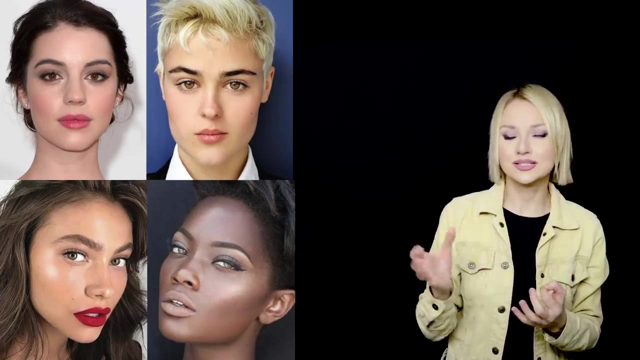 to their appearance. if we talk about lightness and darkness scale, Many of them can have hazel eyes, A little bit more dull appearance. So again, they can be on a softer side if we talk about soft and bright coloration. right, So they can be less understandable and slightly muddy, but they can. 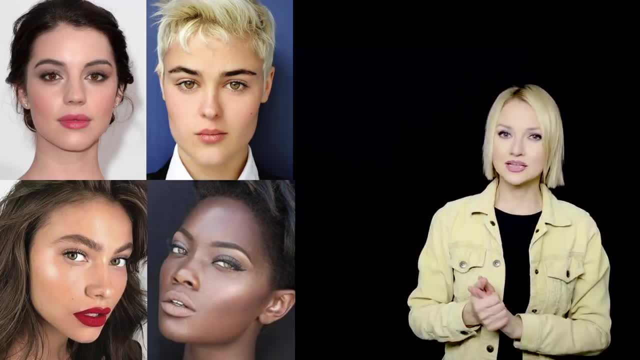 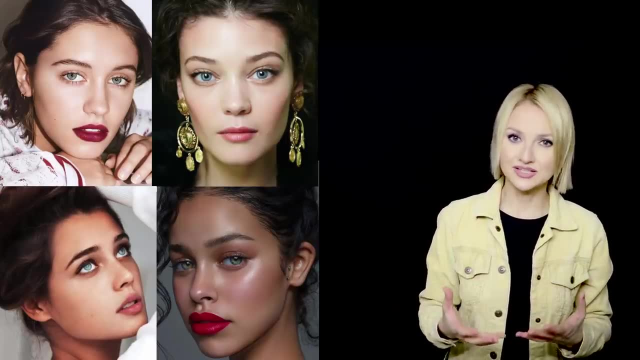 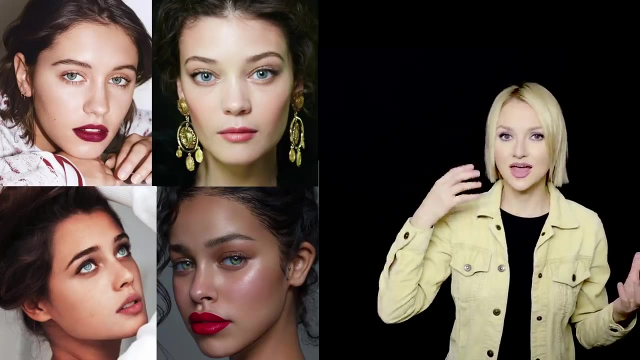 be just darker on the darker side, closer to the brown color, And if they have clearer eyes they can have brighter blue eyes, brighter green eyes, brighter gray eyes, lighter gray eyes Because see light eyes, clear colors of light eyes, especially if they have dark hair and they're 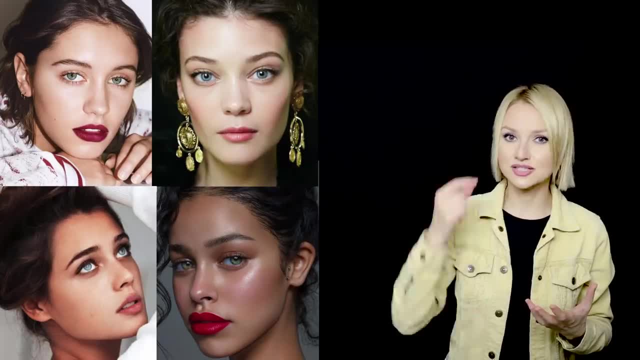 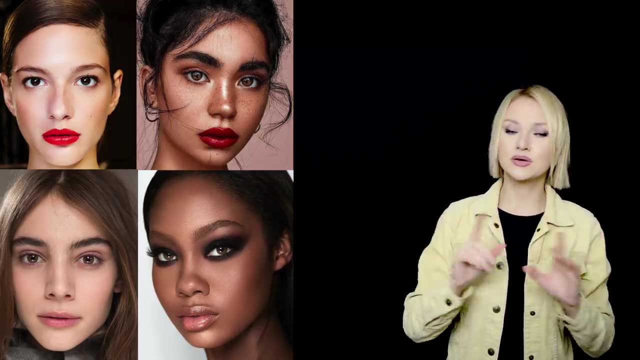 skin can be darker. That creates also a lot of contrast, especially they have the frame around their iris. So again, it's a combination of many things, I know, but we are only looking at one thing today. Or again they can have their clear brown colors, very intense, beautiful, like a glass. 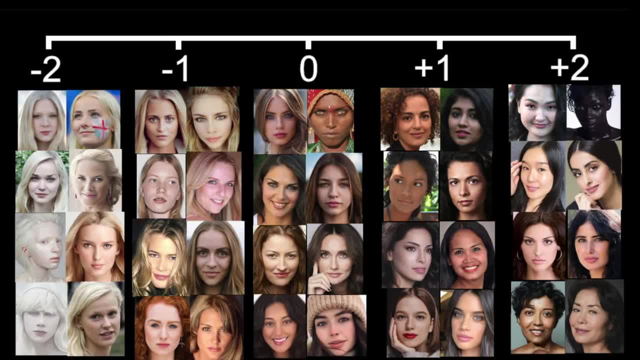 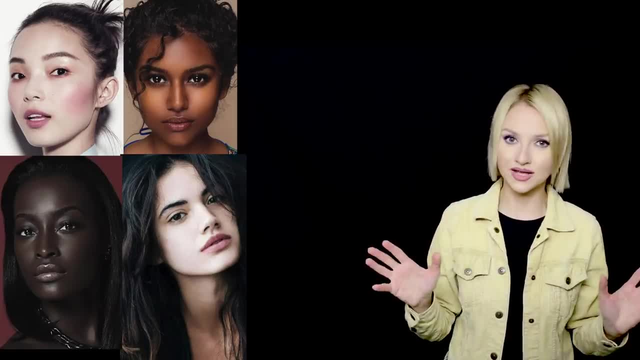 In plus two contrast category: most women have black eyes or very, very reddish, intense brown colors, which is very clear, very understandable and very contrasted with the whites. Their eyes just pop right away. They have a lot of contrast. They have a lot of contrast. They have a lot of. 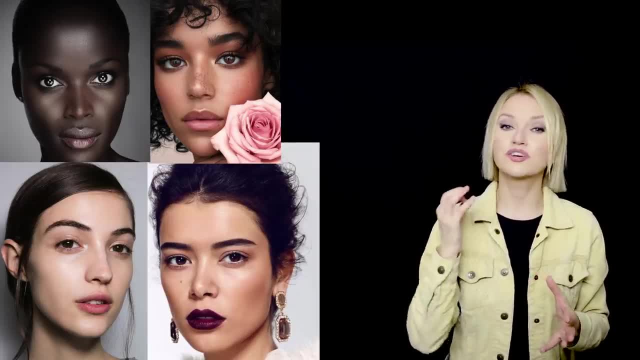 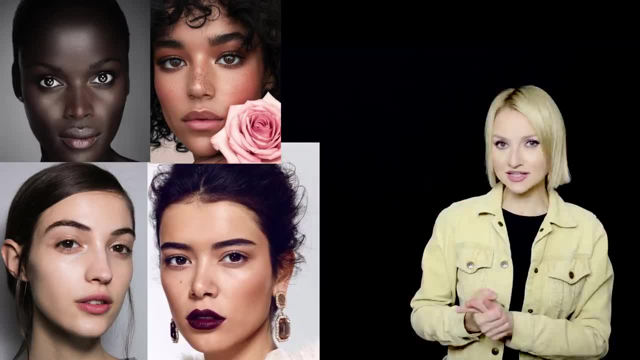 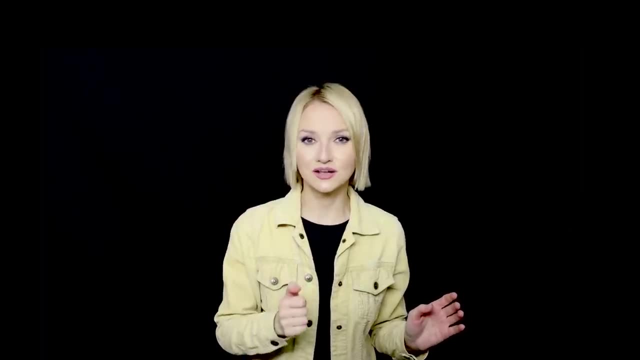 or very light and pale but still pretty clear skin. So what you can do- there are loads of objects in your house- probably Just go to the window, get the mirror or just make a selfie. Just find something that you think is close to your eye color, preferably without any patterns. 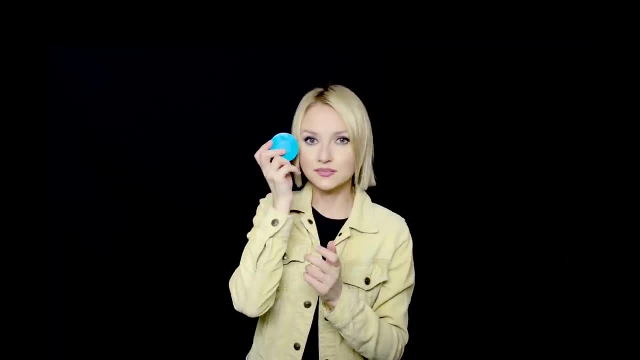 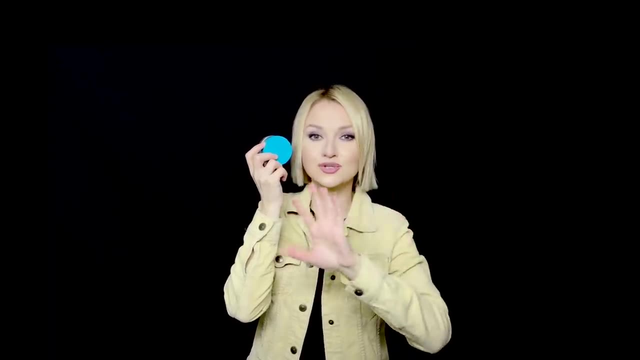 because patterns would really distract you. Get just something, something clear. just put it close to your eye, as close as possible, without any makeup, by the way. Just come to the mirror during the daytime. Better if sun is not shining on you, especially in the evening or early morning, because the sun has. 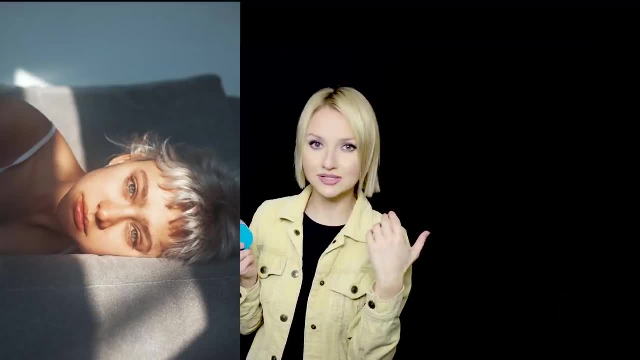 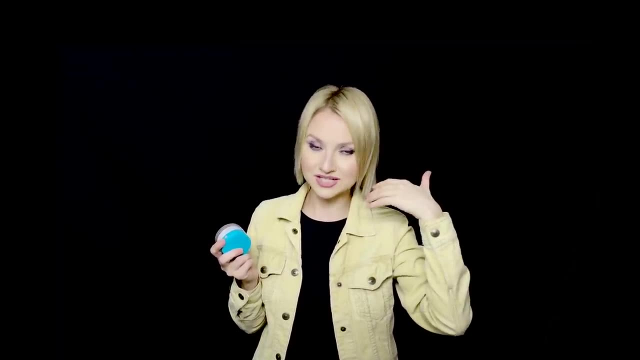 very yellow color to it. It will add some yellow color to your eyes and you will feel like you're warmer, even if you're cool. So the best light would be daylight and if the sun is not shining to your face like crazy. So you're getting that color. you make the photo, then you're getting 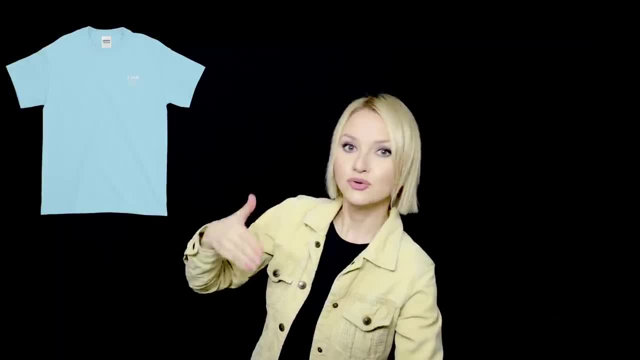 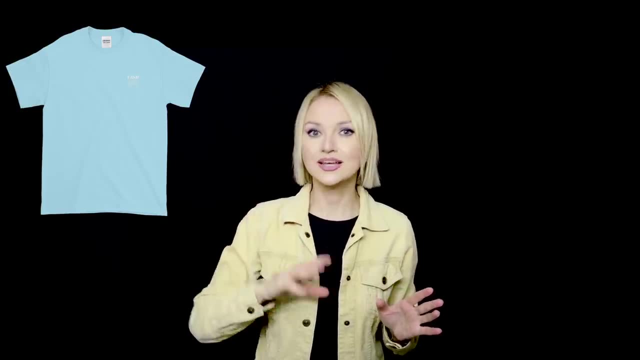 something else. You make the photo and you continue doing that. I think best thing is close Just one solid color, Even if it will be hard for you to understand the first day. next day you get back to those pictures you will understand so much more about yourself. 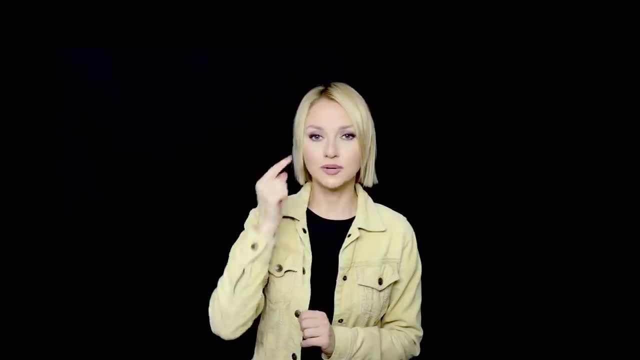 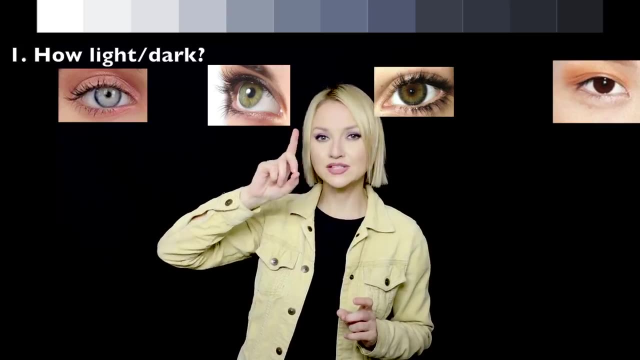 and about your eye color. So how do you analyze that? Compare those two colors and first question you have to answer: is your eyes lighter or darker than this thing? So you have to place your eye color somewhere on the darker, so lighter scale. So it's in the middle. 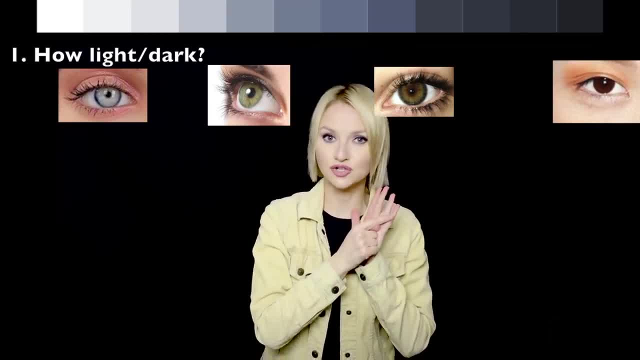 great. Just put a check mark. It will be really helpful for you in the future, especially when you're in the middle of the day. So if you're in the middle of the day, you can put a check mark. It's really helpful. Lightness and darkness is important Every time. 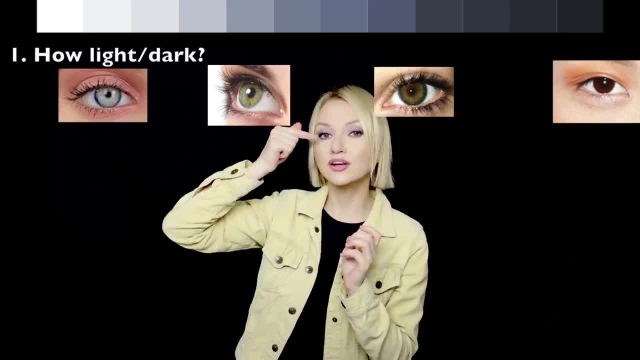 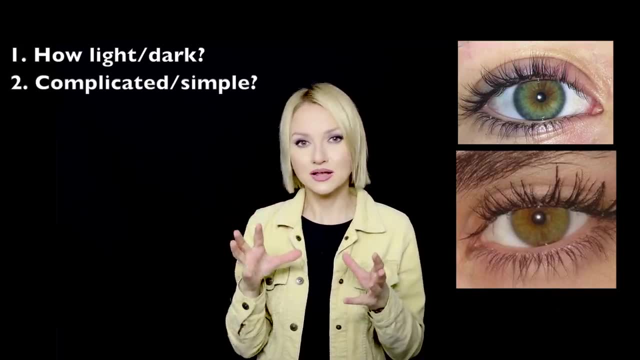 you're comparing to the new color. answer that question first: how lighter your eyes are or how darker your eyes are comparing to that thing. Then the second question: ask yourself: is your eye color complicated? Does it consist of many colors Or is it one plain color? 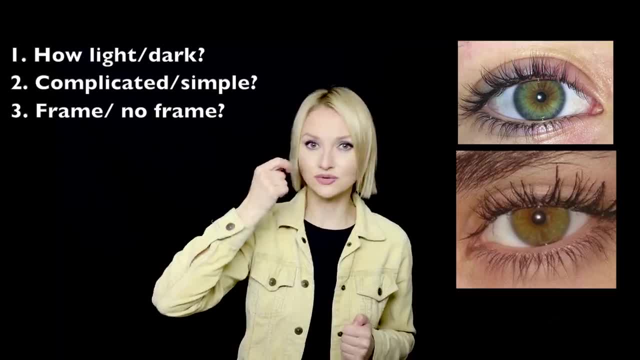 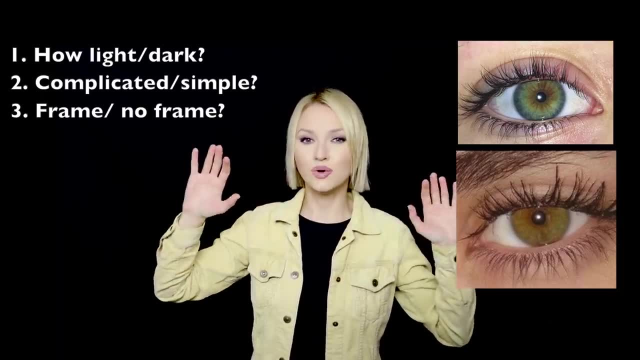 Then another question to answer. do you have dark frame around your iris, Yes or no? If yes, it's more contrasted. If no, then it probably blends to your whites. If your eyes are on the lighter side, that's important. If you're on the darker side, 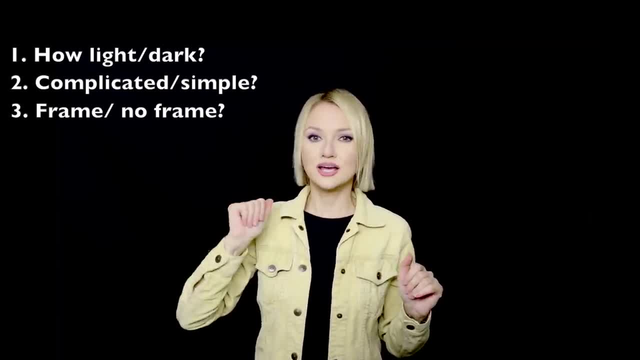 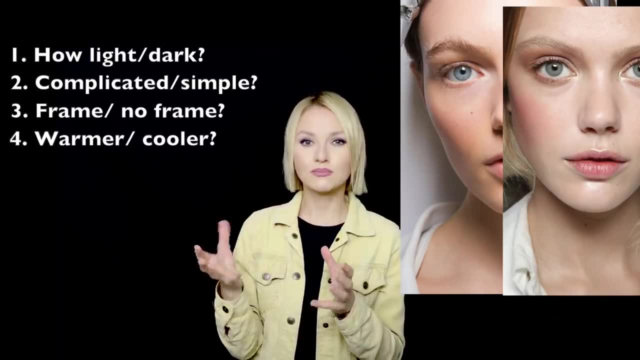 probably it won't change that much. Then you have to understand: is it on the warmer side or the cooler side? So the best thing would be, like I did: Take something blue, Take something bright blue and more dull blue in the middle of darkness and lightness, And just check how. 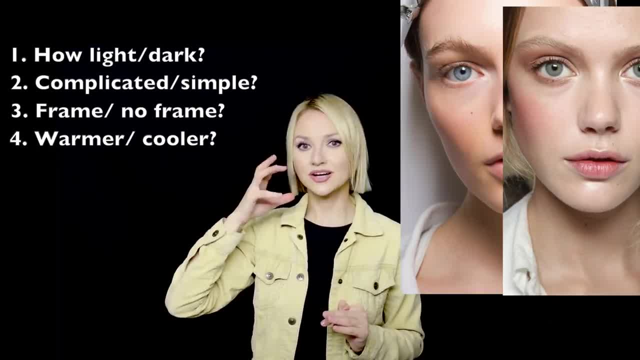 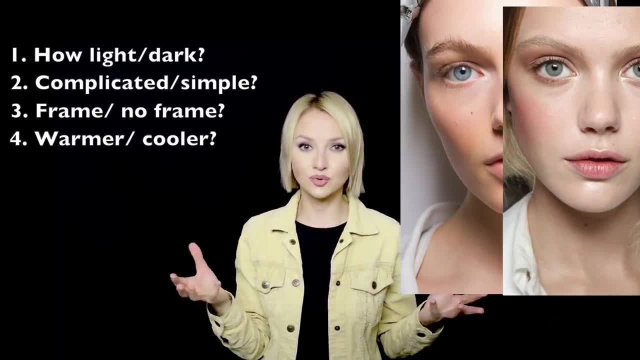 your eyes, look comparing to that thing, And then you will clearer understand. let's say, if your blue eyes, maybe they're on the greener side and you never knew that because you always thought that they are blue and cool. But then when you compare that you 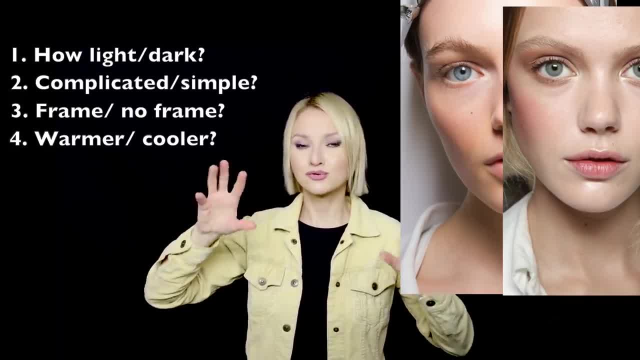 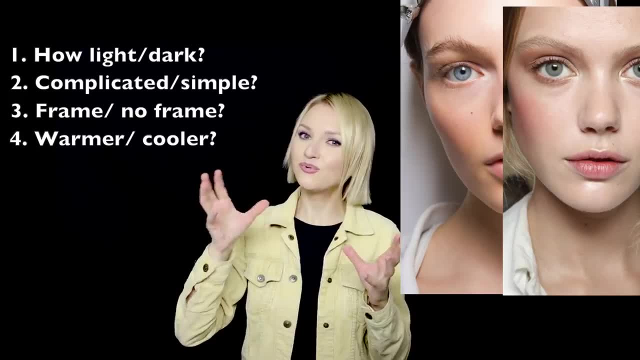 You will see that slight yellowness is coming through, Slight warmth is coming through, And then you will try to pick something from your home that is actually also blue, but also on a warmer side blue, And you pick it up and you compare it to your eyes. 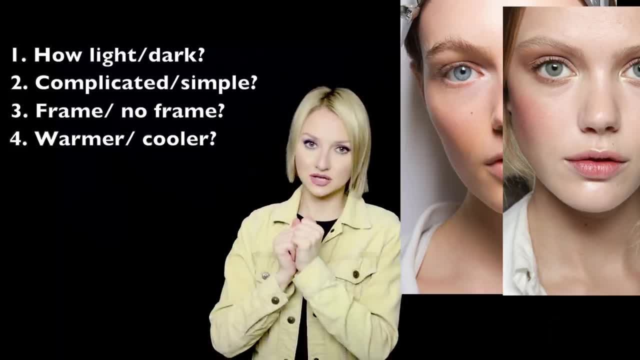 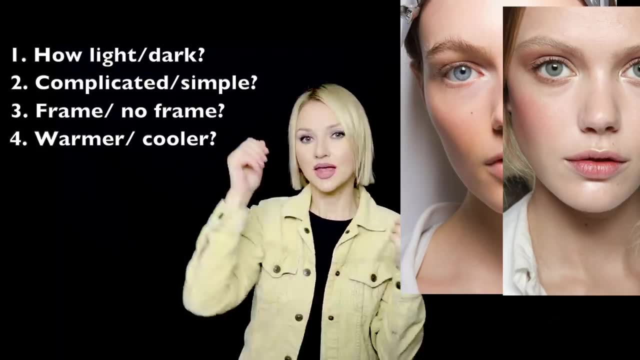 and it will match, let's say, completely. And then you analyze this color. Just analyze this color that matches your eye color. Analyze what is this name it Compare it to other colors in your home and say if it's dark or light or it's somewhere in the middle. 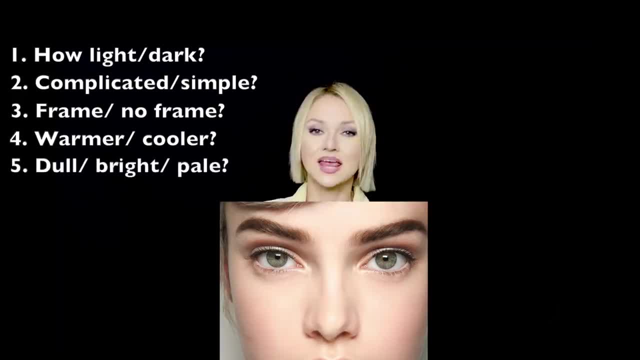 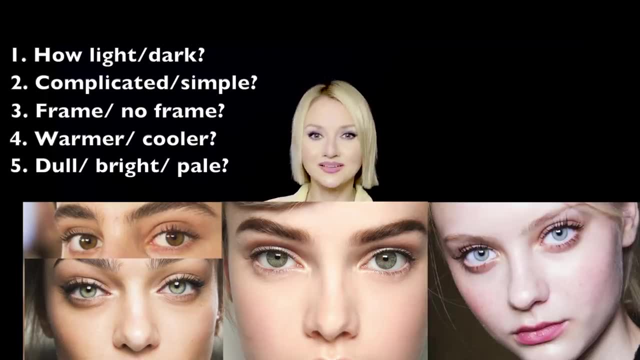 And say if it's on a warmer side or on the cooler side, And say if it's dull color, have some gray colors in it, not very clear, or it's very bright color, Or maybe it's very pale color with added white to it. 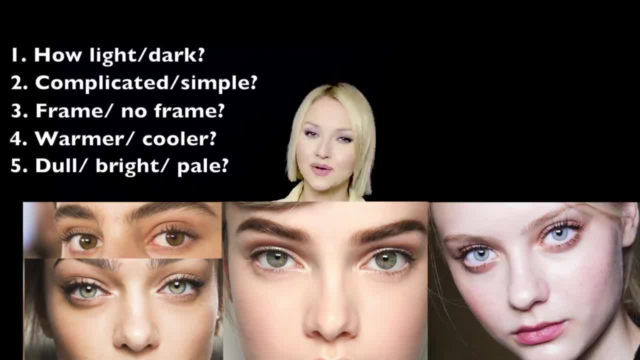 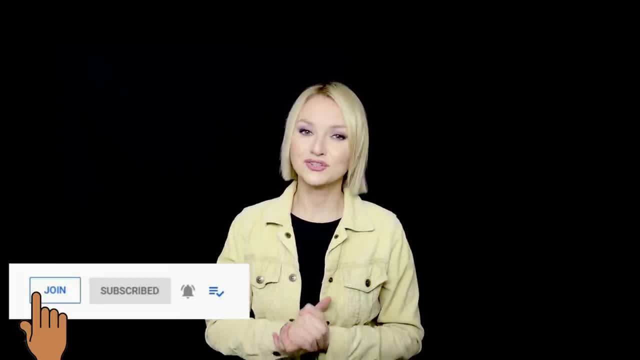 Probably it doesn't contain any gray color. So make this homework and I will wait you in my next video. Thank you so much for watching, guys. If you want to support my channel, you can either click the join button here on YouTube and become my sponsor, or you can subscribe on my Patreon. 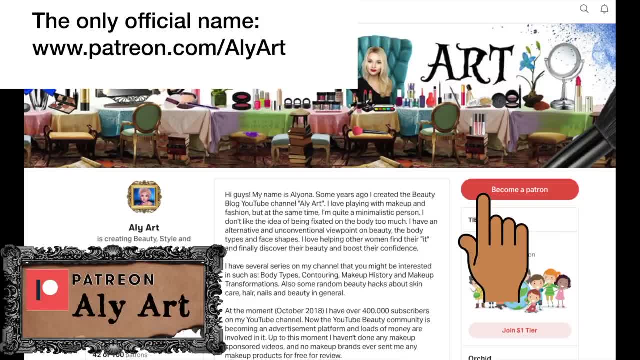 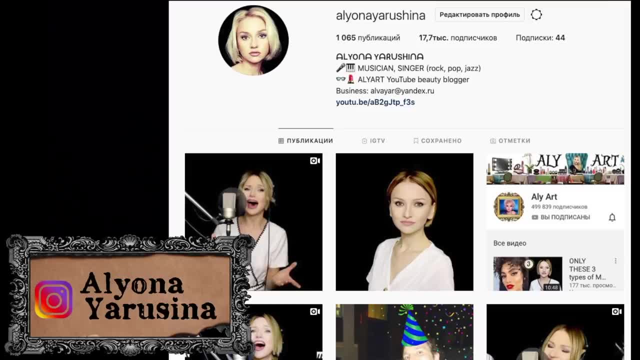 There will be some exclusive videos for you guys And also early access- And please make sure this is the only correct name for my Patreon. You can subscribe on my Instagram for just random stuff from my music and from my makeup life. You can also subscribe on my Pinterest.